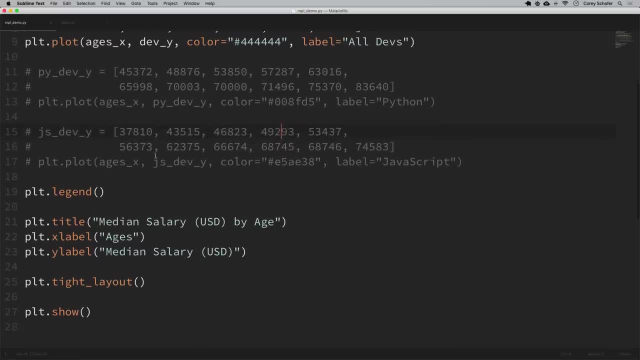 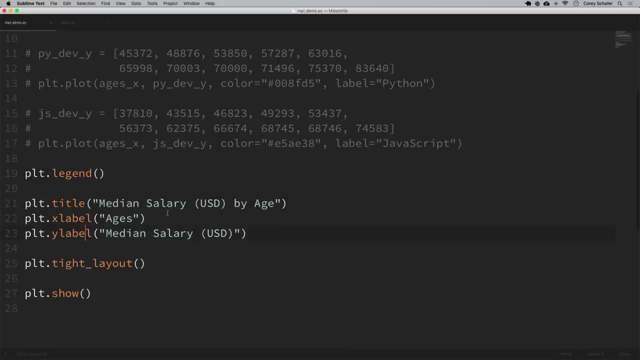 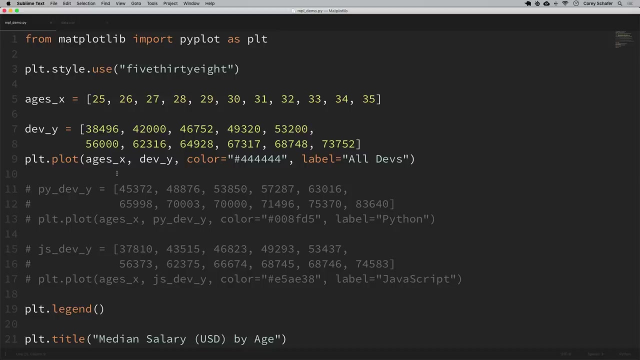 This is for JavaScript developers here, But I've got those commented out for now. We are also putting a legend on our plot, giving it a title, x and y label, giving it a tight layout which just helps with the padding, And then, lastly, we are showing it. So, when we plotted our data in the 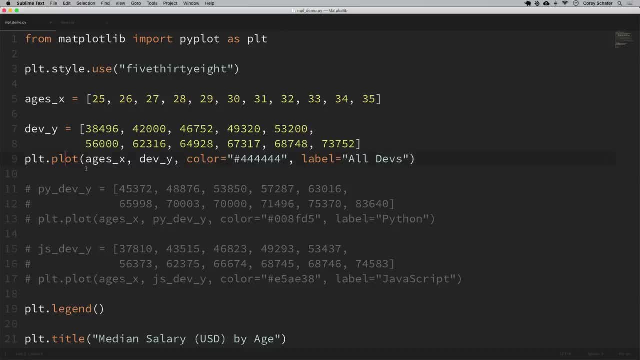 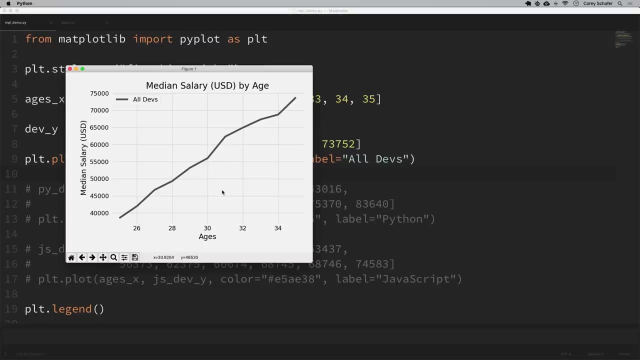 last video we used this pltplot method And when you use the plot method it will use a line plot by default. So if we run this, then we'll see something kind of similar to what we saw at the end of the last video, So we can see that we get a line plot here for the median salary of developers. 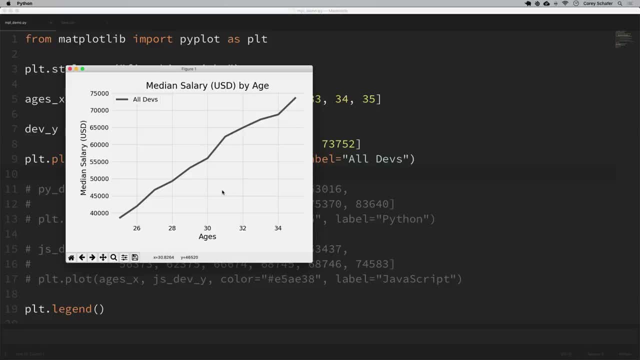 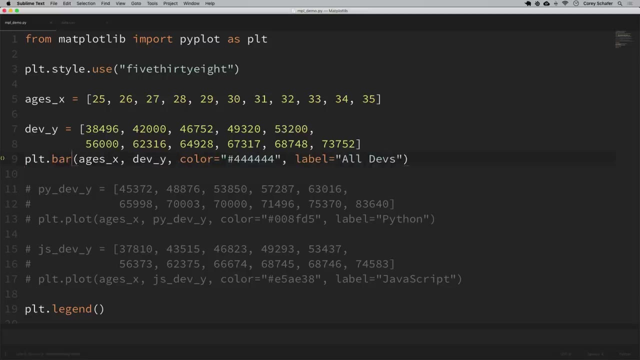 And again, this is some data that I took from the annual Stack Overflow Developer Survey. But let's say that we wanted to show this as a bar chart instead. Well, to do that, we can simply use the bar method Instead of the plot method. So if I just change this to use bar instead of plot, then we'll have a 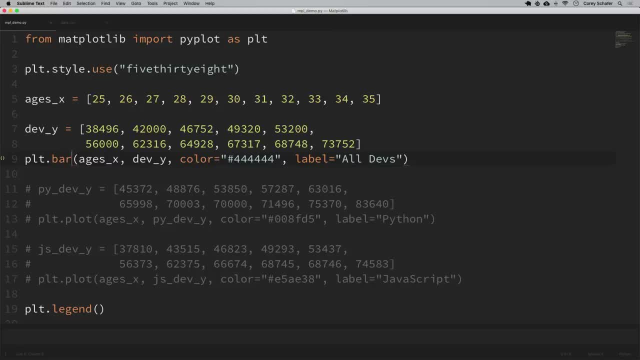 bar method or a bar plot, sorry. And just like that plot method we can pass in our x values first for our x values and the y values for our y axis, And additional parameters here can be passed in as well, like color and label. So I'm just going to leave that as is, just like it was with the plot. 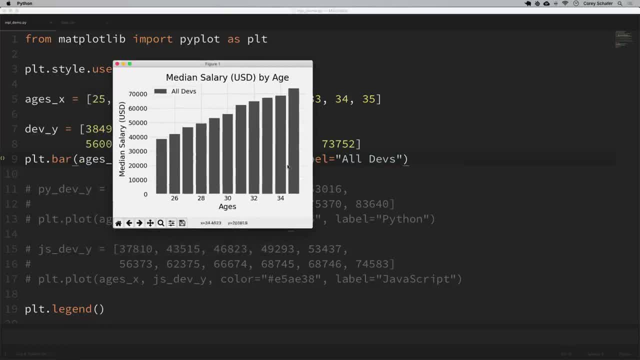 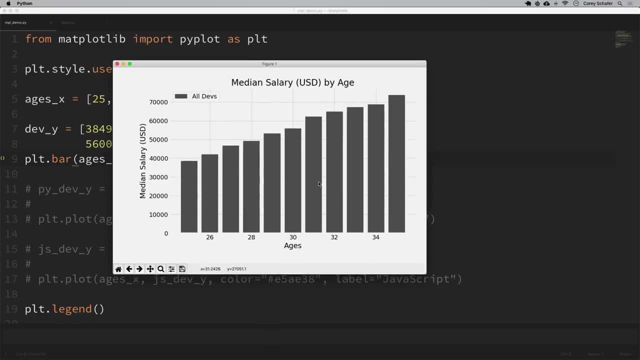 method And if I run this, then we can see that now this is plotting our data and it's represented as a bar chart instead. Okay, so that is plotting the data for all developers who answered the survey. So, like I said, I also have the data for Python. 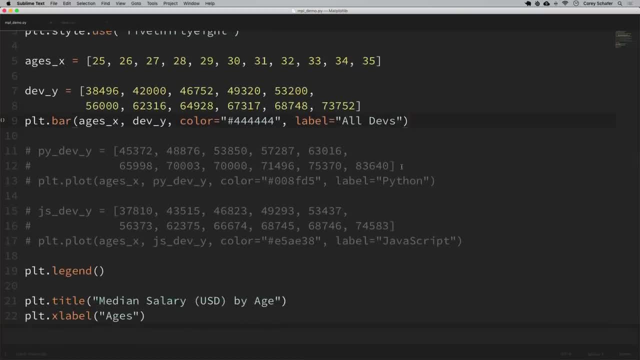 and JavaScript developers as well, And right now those are commented out. So what if I wanted to include those in our bar chart? Well, first of all, you can mix and match some plots. So if, for some reason, you wanted the Python and JavaScript data to remain as line plots, then you can. 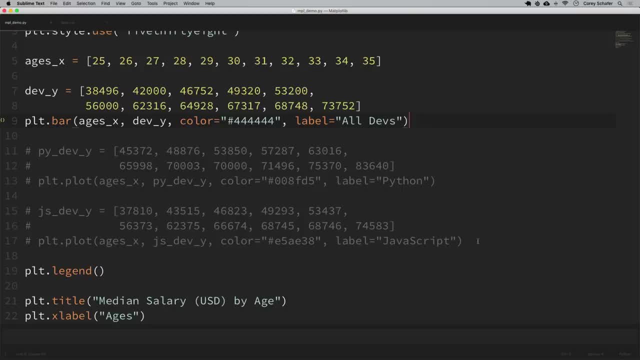 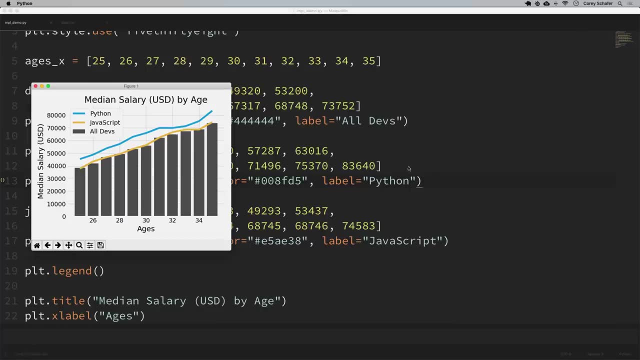 overlay that onto our bar chart, Then we could simply uncomment out our code here and we could just run these as plots And that will actually overlay line plots on top of our bar plot. Now that doesn't make much sense in this situation, but depending on your data, you might find that. 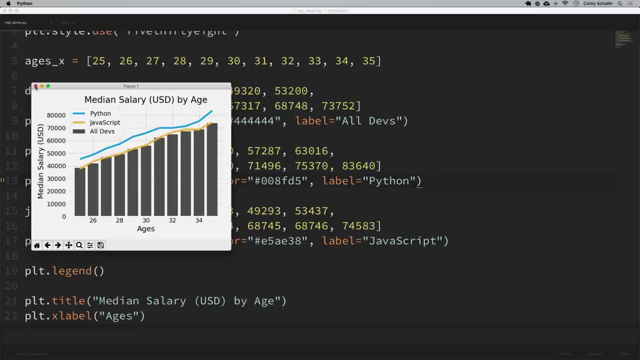 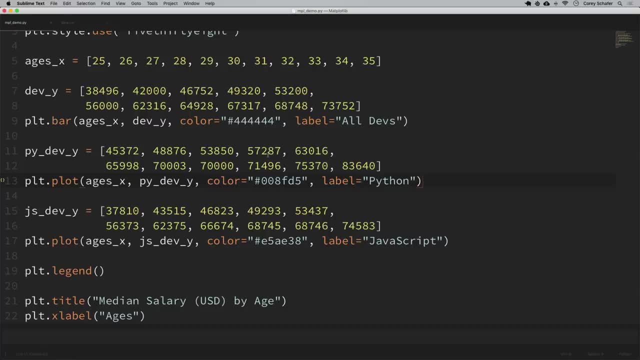 useful. Okay, but what if we wanted to include these in our bar chart as bars, side by side with the other data? So you might think that we could do this just like we did our line plots, and just run those using the bar method as well, But that's. 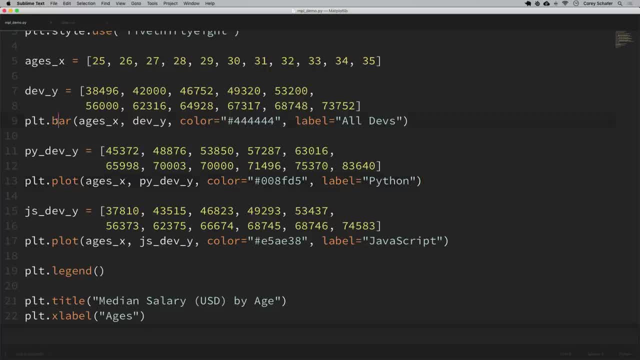 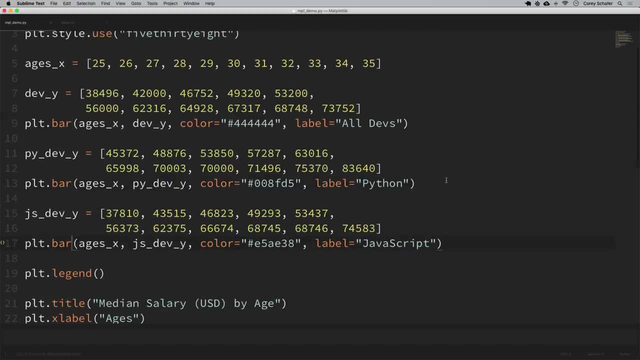 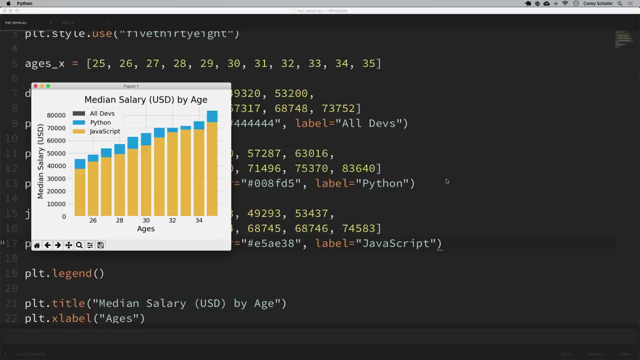 actually going to give us some issues. So let's try that real quick and see what that does. So I'm going to change these to use bar, so pltbar. So I'm going to run that and we can see that this doesn't quite look right. We can't even see the data for all of the developers and the data for 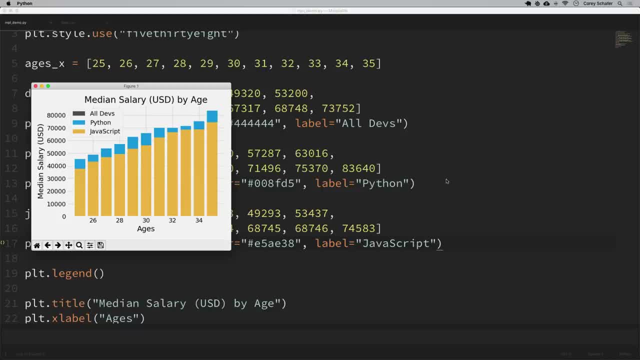 Python and JavaScript is overlapping. So how can we do that? Well, we can do that by using the X values. So let's say we put these side by side, because right now they're just all stacked on top of each other. So we can do this by offsetting the X values each time we plot some data. Now, 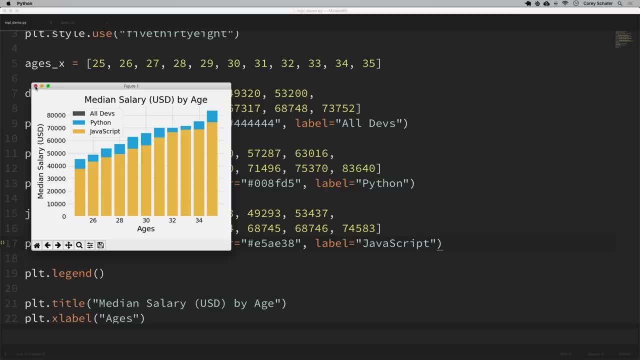 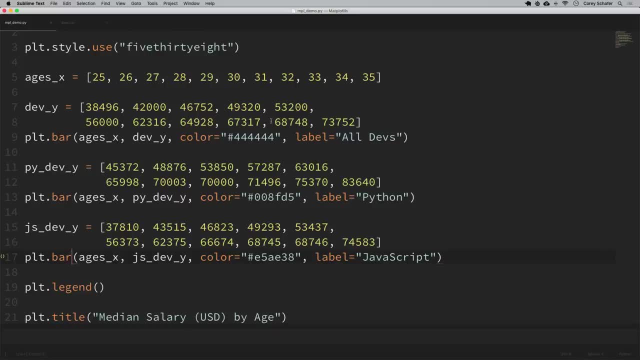 I actually think this is a lot harder than it should be. It seems a bit hacky in my opinion, but this is just how we have to do it. So to do this, we're going to have to import numpy and use that to grab a range of values for our x axis. Now, if you've never used numpy before, then don't. 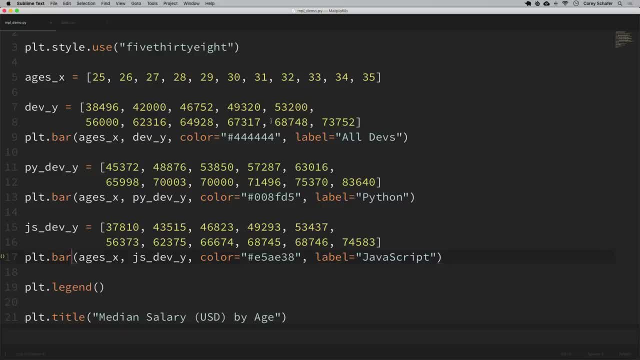 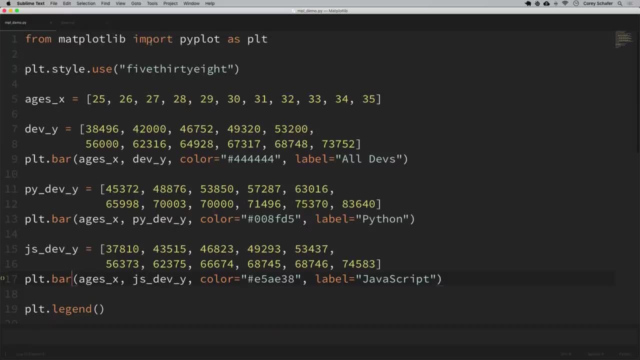 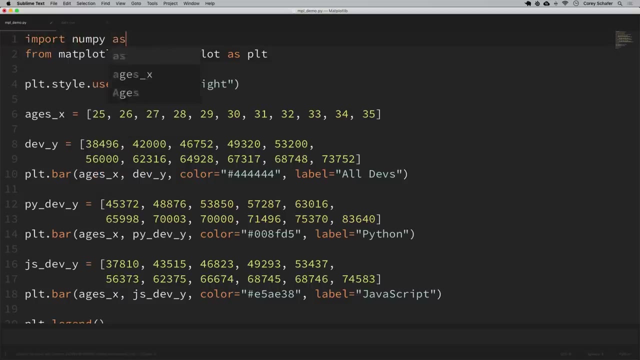 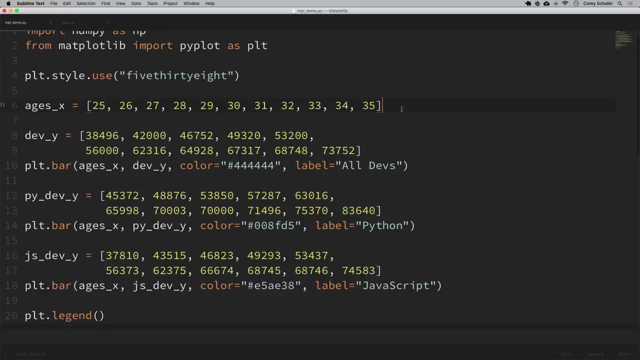 worry too much about it. It's just going to use one simple function. So we're going to do that. So I'm going to say import numpy and I'm going to import that as MP. That's a convention there when using numpy is to import it as MP. And now, below our X values, here where we have our ages X. 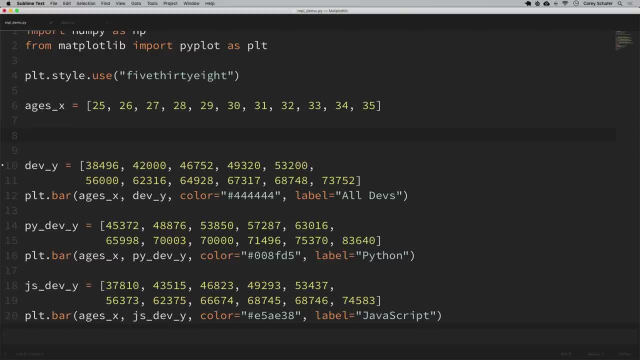 I'm going to create a range from these values. So I'm going to say X underscore indexes and I'm going to set this equal to MP dot a range, And I'm going to pass in the length of our ages X list here. And what that's going to do is it's going to create a variable called 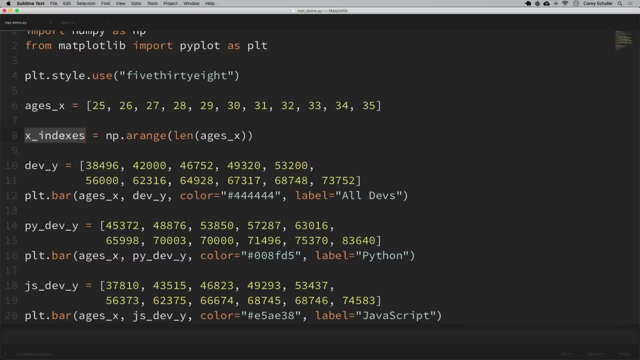 X indexes, And that is an array of values, And those values are going to be a numbered version of our X values. So basically, it's a lot like having a list with an index starting at zero and counting up to our last value. So I'm going to set this equal to MP dot, a range, And I'm going 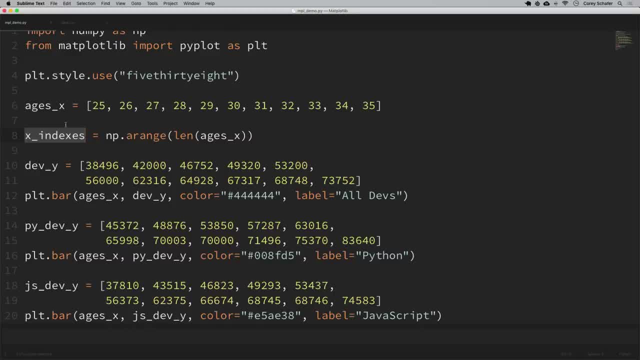 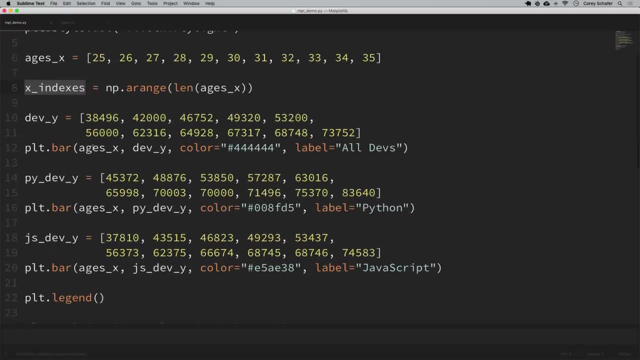 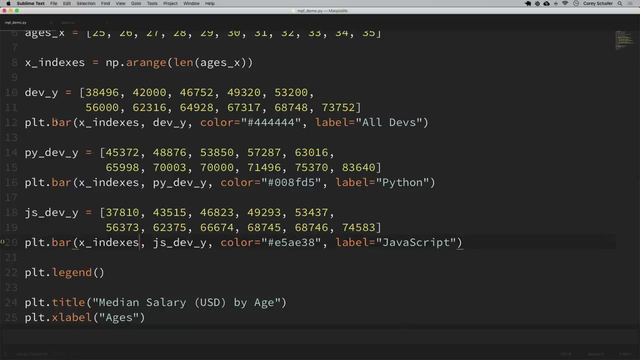 to copy that, And instead of using our ages here, I'm instead going to use those X indexes. So I paste those X indexes into each of our bar methods here. So if I were to run this right now, then it would look very similar to what we had before, But now we're just using those indexes instead. 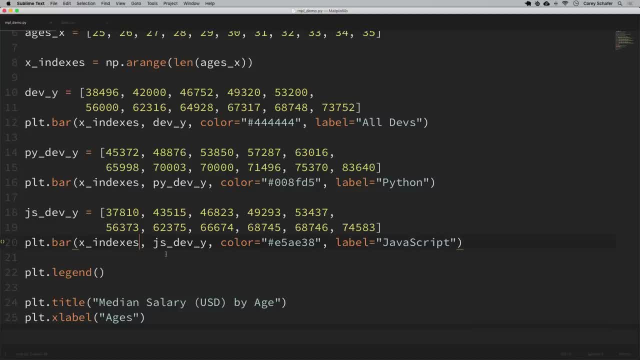 But now that we're using these indexes, we can actually shift the location of these by adding or subtracting to our values here. So, if we think about it, they're all stacked up on top of each other right now. So let's shift. 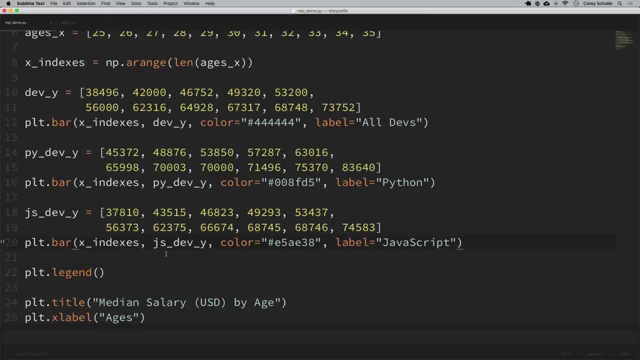 our first bar to the left and the second bar to the right. But how far do we actually want to shift these? Well, we want to shift them by the exact width of a bar. So, to do this, it would be nice if we specify an exact width for our bars, so that this is explicit. I believe that they have a 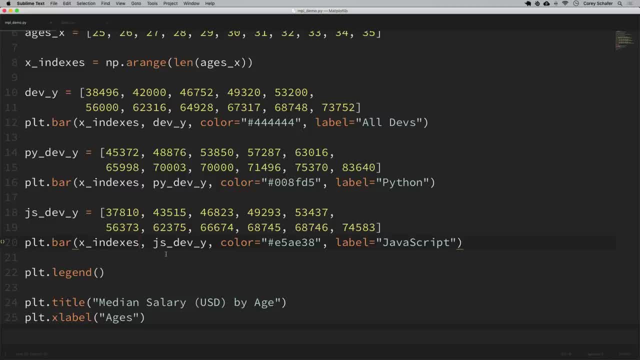 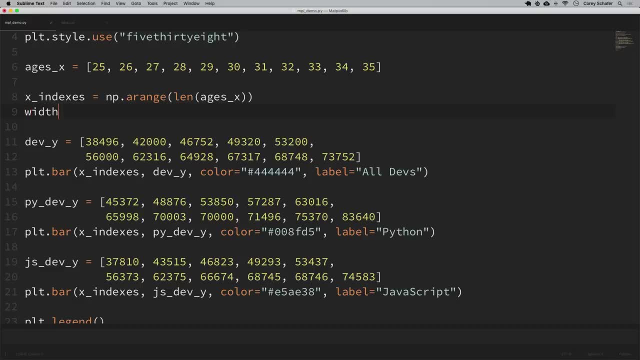 default width of a bar. So we're going to set this equal to MP, dot a range, And I'm going to set this to a width of like zero point eight or something like that. But just to be sure, let's create our own width variable. So up here underneath X indexes, I'm going to create a width. 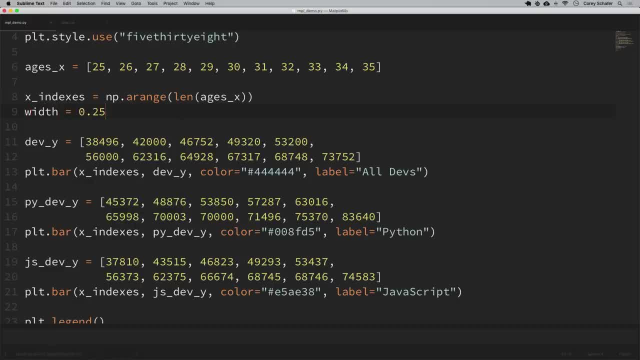 and set this equal to zero point two five, And I think the default of zero point eight is going to be a little thick with three bars being side by side, So I think zero point two five would be good here, But you can experiment with these different widths if you'd like to get different looks. 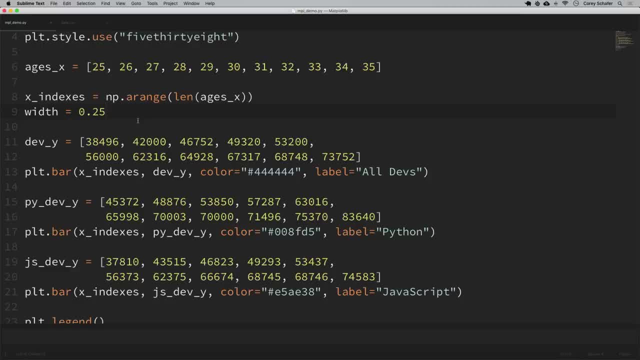 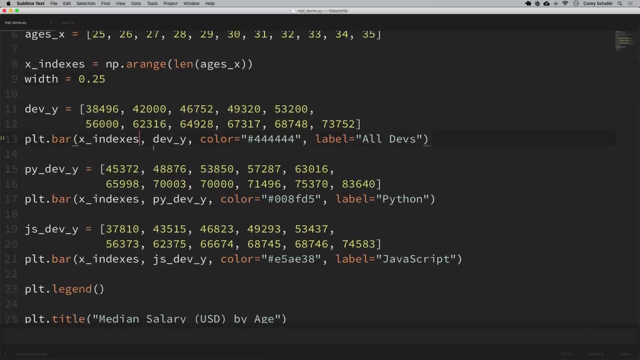 depending on your data. So what we're going to do is we're going to add a width. Let's subtract that width from our first plotted values And we'll add that width to our last plotted values And that should shift those bars to all be side by side. So with our first bar plot here, which is right here, we are going to 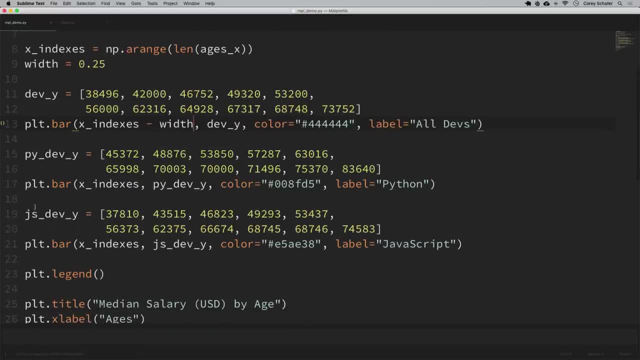 say X indexes minus width, then for our second bar chart we're not going to do anything because that's going to be in the middle. And then for our last bar chart we'll say plus width, since we want that to shift to zero point two five. And then for our second bar chart, we're not going to do anything. because that's going to be in the middle. And then, for our last bar chart, we're going to say plus width, since we're going to say plus width, since we want that to shift over to the right. And lastly, before we plot this, 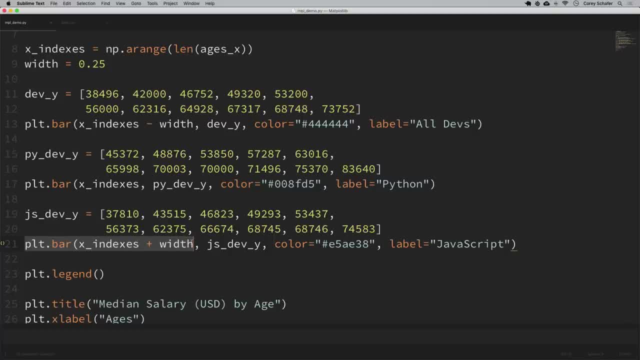 we're actually going to need to tell our plot that we want the width of the bars to be equal to the width variable that we just created, And we can do that just by passing in a another variable here. So right before color, on all these, I'm going to add a width. oops, let me spell that right: width equal to width. 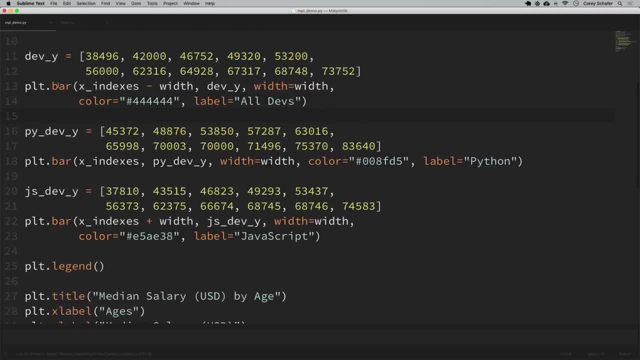 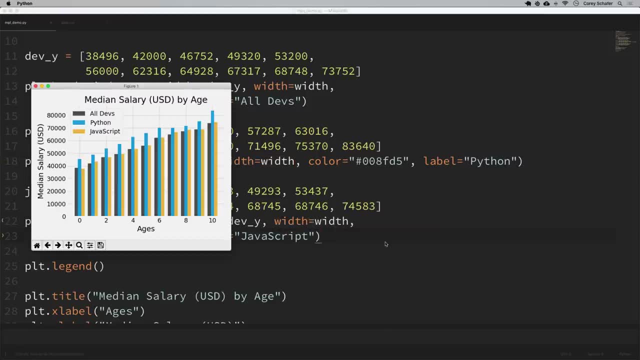 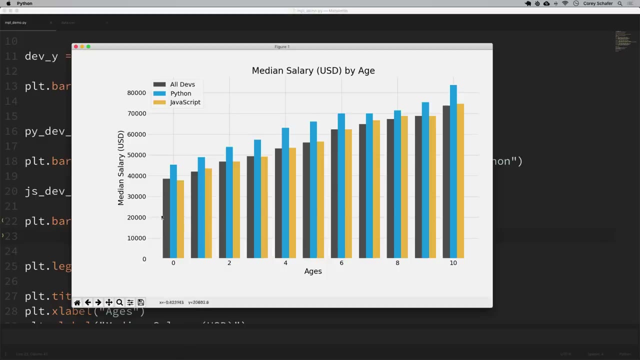 And I did that for all three of these bar methods. So width equals width here, here and there. So now that we've done that, if we run our code here, then now we can see if I make this a little larger here. we can see that now our bar chart has these all lined up side by side instead of. 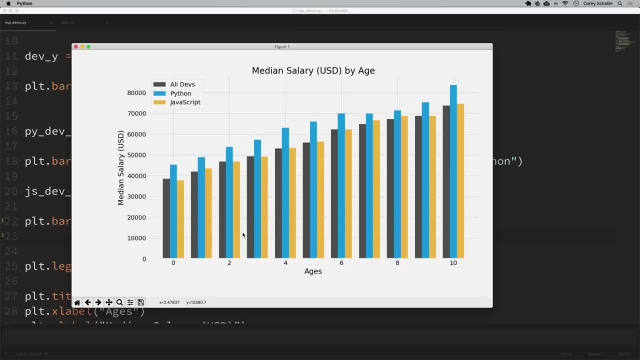 being stacked on top of each other like they were before. Now, if you have more or less bars that you need to fit side by side, then you'll have to adjust the offsets accordingly for the number of bars that you have. The way that I did this was with three, but if you added another bar, 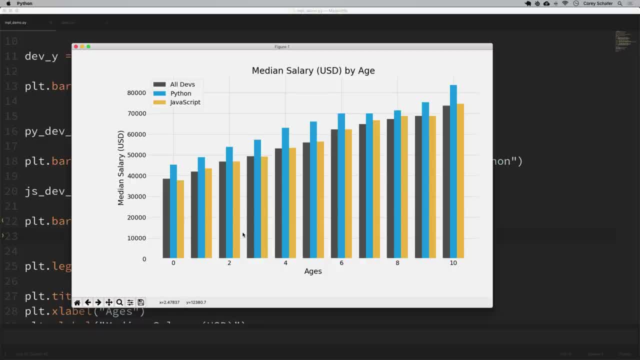 then you'd need to do an offset with the width added twice, and so on. Now, also, if we look at our x-axis down here, we can see that we no longer have the age ranges that we had before. It's using the indexes, since that's what we needed to do our offset. So to fix this, let's go back to 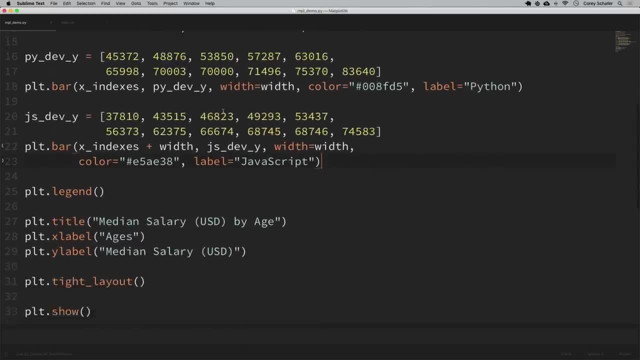 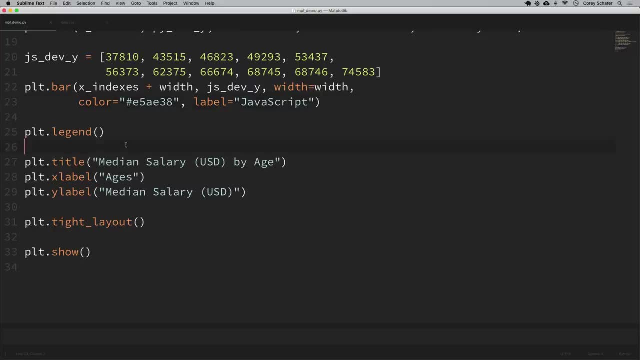 our code. So I'm going to shut that down. And down here towards the bottom, we're going to need to use an xtix label to change the labels. So right here above the title, I'm going to say pltxtix. Whoops, let me spell that right. So within this xtix method. 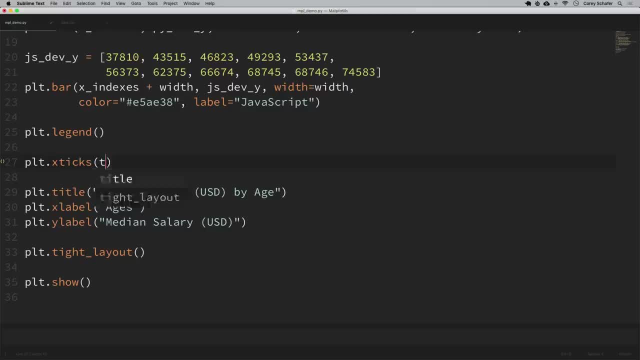 we need to pass in a couple of arguments. So I'm going to say: tix is equal to, and those tix are equal to the x-indexes. Now the labels for those tix are going to be equal to our ages list here. 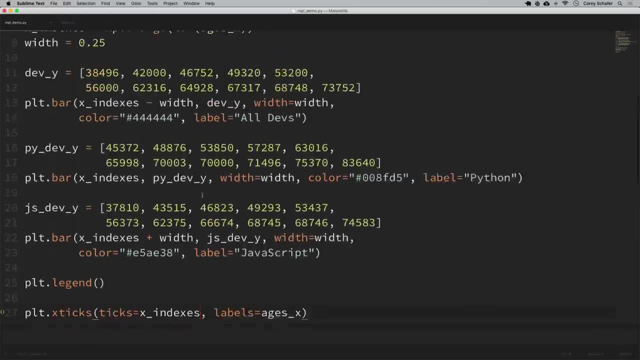 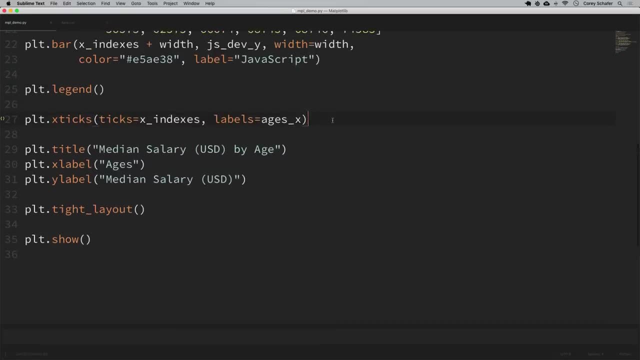 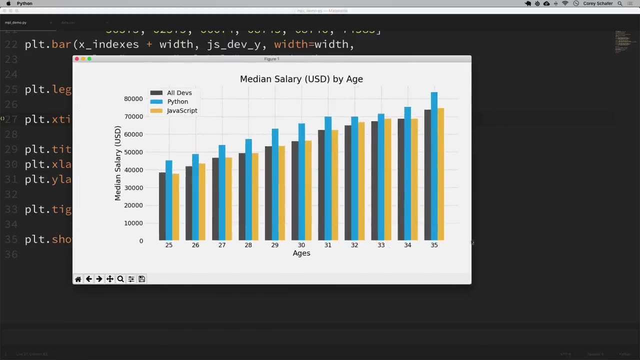 So we are using those x-indexes for the tix and the labels which are all of our ages that we saw before in the last video. We're going to use that for our labels. So now, if I run that, then we can see that now our plot has our x-axis labeled correctly. Okay, so we've looked here at 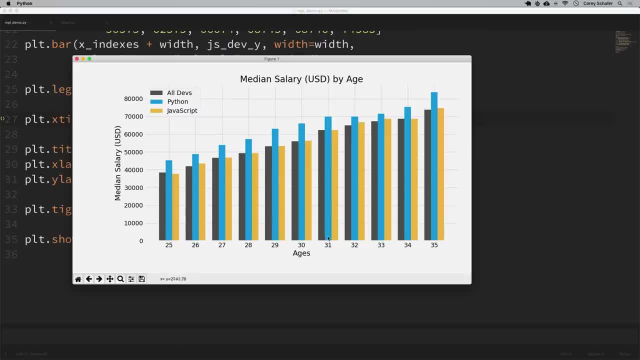 vertical bar charts and how to add multiple different bars to that plot, And in a minute we're going to look at how to create horizontal bar charts. But first I want to load in some data that's more appropriate for a horizontal chart. You usually want to use horizontal bar charts. 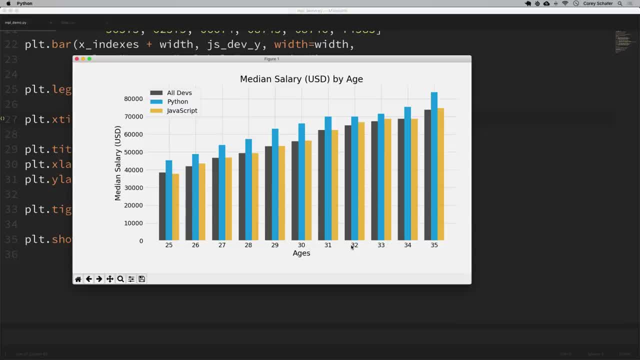 when you have a horizontal bar chart. but you want to use a horizontal bar chart when you have a lot of data and it looks too crowded in a vertical plot, And the data that I want to load in is going to be from a CSV file, So so far we've only used data that has been directly in. 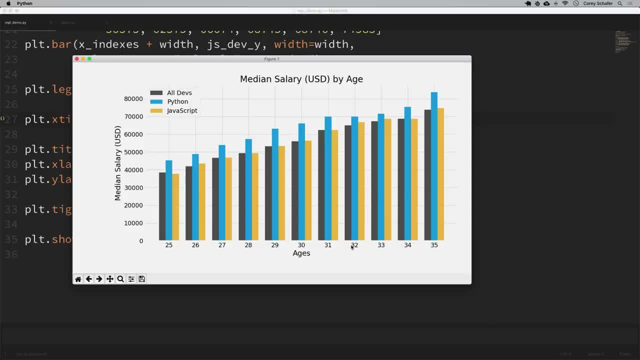 our Python script, But most of the time you're going to be likely using data from external sources like a CSV file, And sometimes you're going to need to work with that data a little bit before it's actually ready to be graphed. So first let me get rid of the data that we've 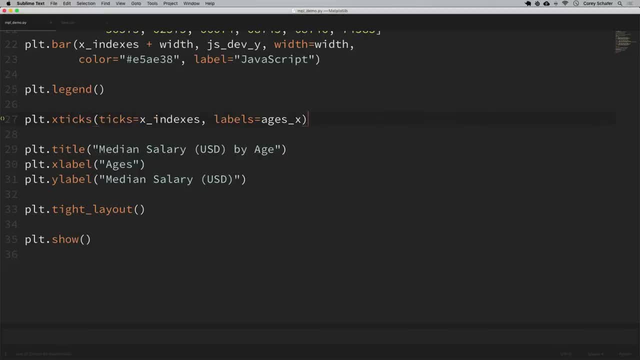 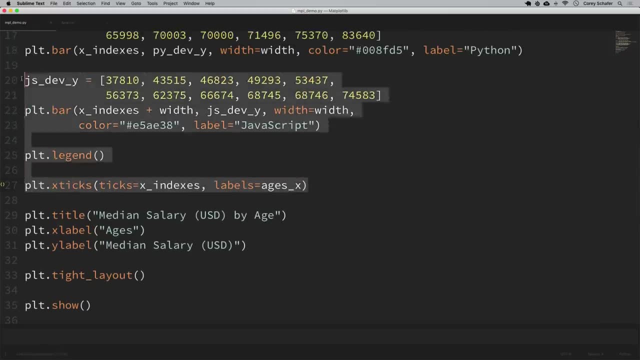 been using so that we can make room for data that will load in from our CSV file. So I'm going to remove, I'm going to remove all the way from our PLT X ticks there. I'm going to go up all the way to our ages and remove all of that data. And for now, 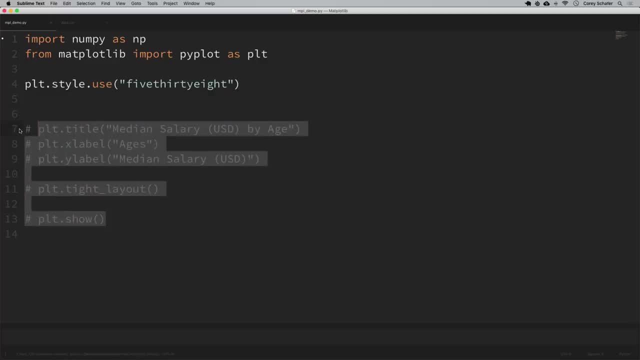 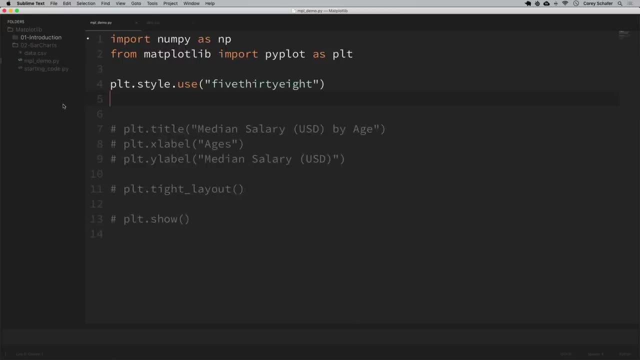 I'm also going to comment out our plot titles and plot show and things like that. And now let me open the CSV file and show you what this looks like. So I have this open here in my current directory And, like I said, all of this is going to be available for download. download, download. 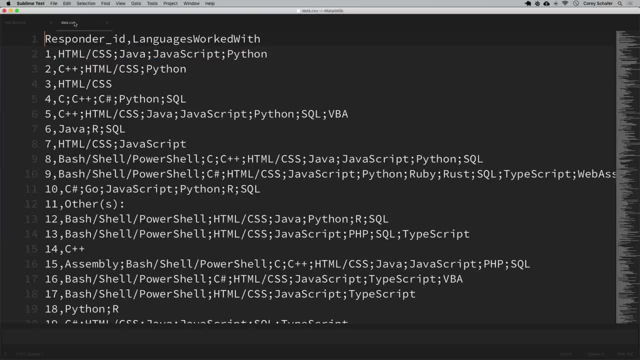 download in the description section below if you want to follow along. So this is the CSV file that I'm going to be loading in here. So this is also data from that Stack Overflow developer survey. but I cleaned it up a little bit and only grabbed the data for the programming languages. 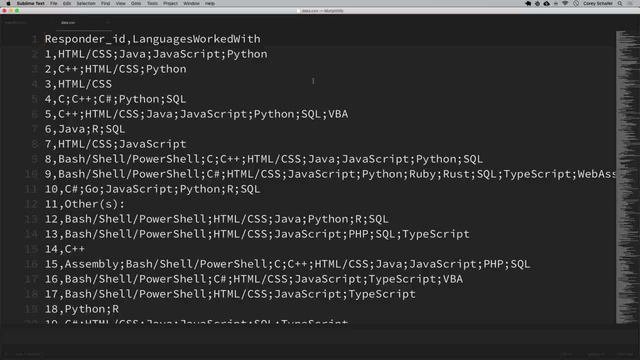 respondents said that they worked with. So we can see that the top line here tells us what information this is. So this first column here is the responder ID. So these are just IDs for each person who answered the survey And this is the responder ID for each person who answered the. 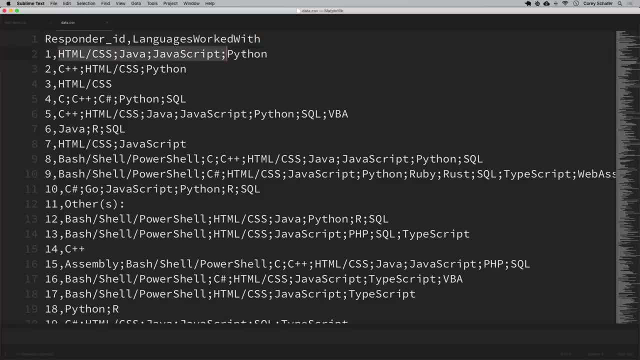 survey And then we can see that the languages worked with These are the languages that that specific person said they knew. So this first person here said that they knew HTML, CSS, Java, JavaScript and Python, And we can see that these languages are all delineated by a semicolon here. 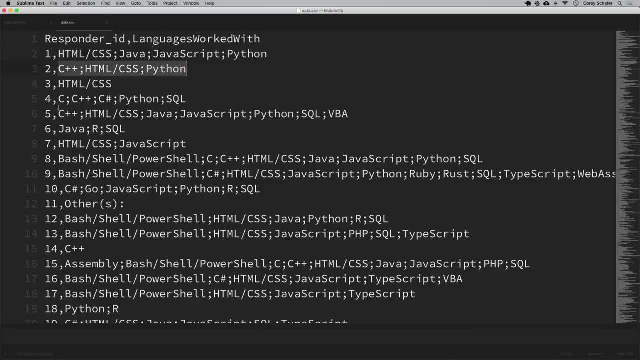 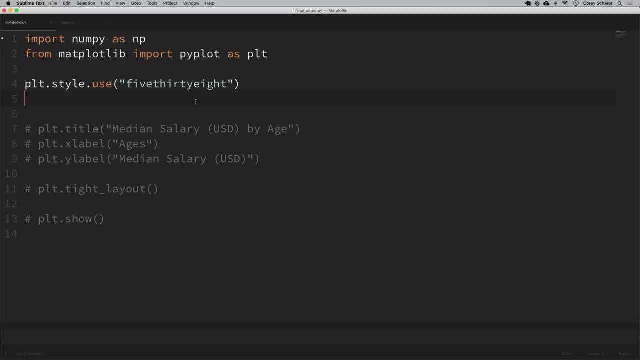 So each line here has all these different languages And using these we can graph the most popular programming languages from that survey. So let me go back to my script here And, like I said, let's say that we wanted to create a bar chart of the most popular programming. 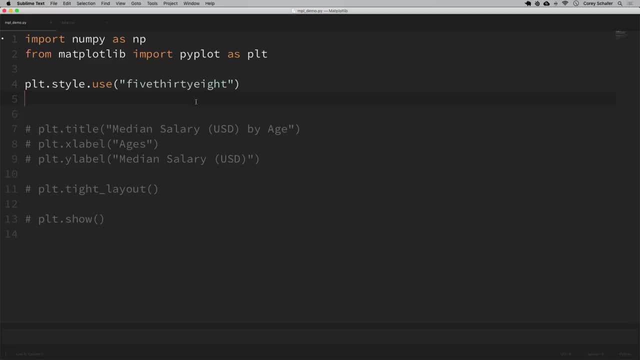 languages that people said that they work with. So first let's grab the data from that CSV file. Now there are multiple ways that we can load in a CSV file. We could use the CSV module from the standard library. We could use the read CSV method from Pandas. We could also use the load TXT method. 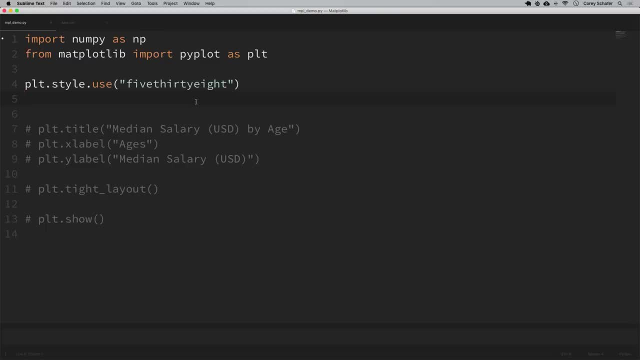 from NumPy. Now, first let's use the CSV module from the standard library, for since most people are probably familiar with that, But then I'm also going to show you a faster way using Pandas, and that read CSV method. So first let's use the standard library to do. 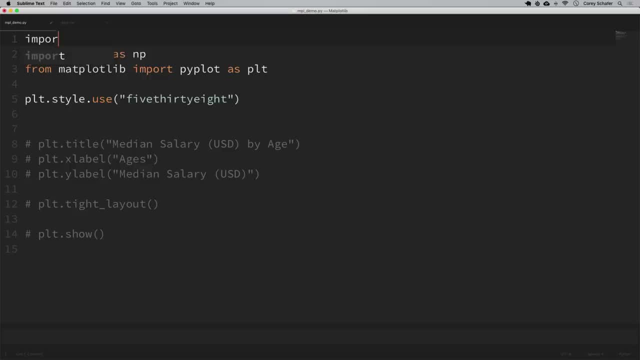 this. So at the top here I'm going to import CSV And now I'm going to read that file using the CSV module. Now, if you don't know how to work with CSV files using the CSV module from the standard library, then I do have a detailed video specifically on that, So I'll be sure. 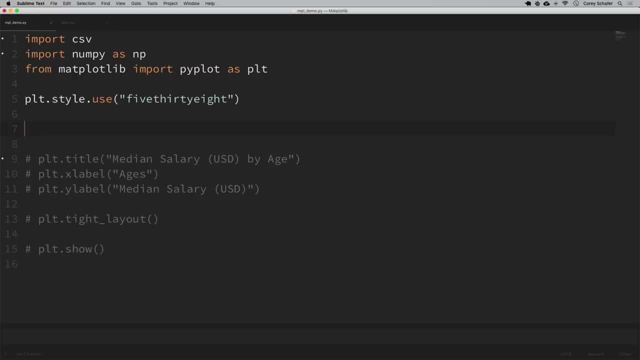 to leave a link to that video in the description section below if anyone is interested. Okay, so the way that we can read this in is I can say with open and we want to open. that file was called datacsv And it's in the same directory as the script, So I don't have to specify a full path. 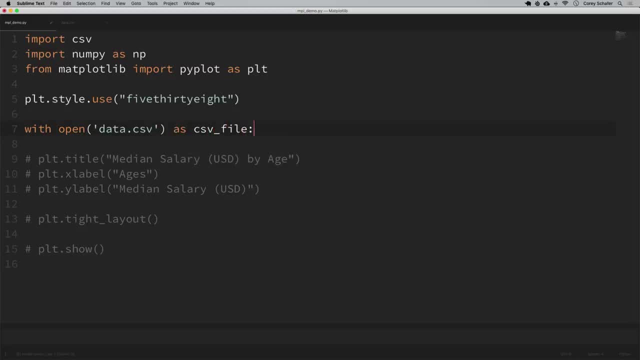 And now we can just say as CSV file, And now we can use this CSV module to read this in. So I'm going to say CSV reader is equal to, and I'm going to use the dictionary reader method from the CSV module to read in the CSV data The dictionary reader actually makes. 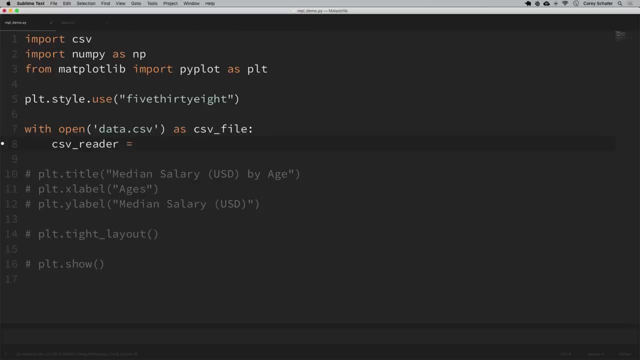 a dictionary where we can access the values by key instead of by index, And I find that pretty helpful. So to do that, that is csvdict reader, And now we just want to pass in that CSV file. Okay, so now we should have that CSV data in our CSV reader variable And this is an iterator that. we can loop over Now. I don't want to loop over all of these right now, but I do want to loop over all of these right now, So I'm going to go ahead and do that. So I'm going to go ahead and do that. 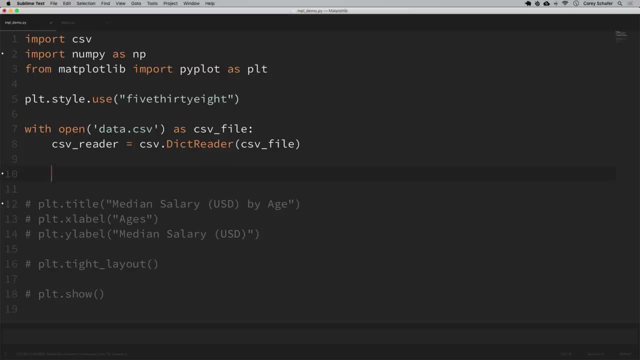 Now, I don't want to loop over all of these right now, but I do want to loop over all of these right now because I think there are like 90,000 rows in that data there. So instead let me just print out the first row, so that we can kind of see what this looks like. 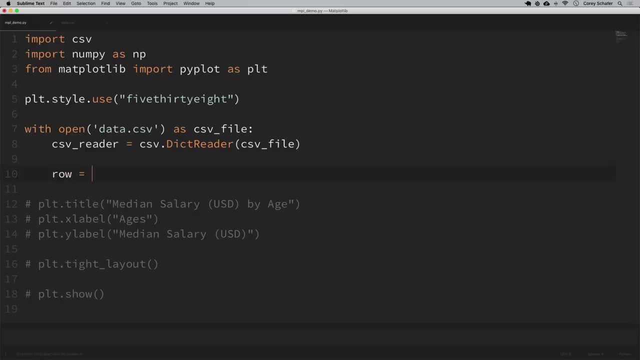 And I can grab that first row by saying: row is equal to next CSV reader And that will grab that first line from that iterator And now let's print that out. So I'll print out row. So if I save that and run it, let me make my output a little larger here. Okay, so we can see that this. 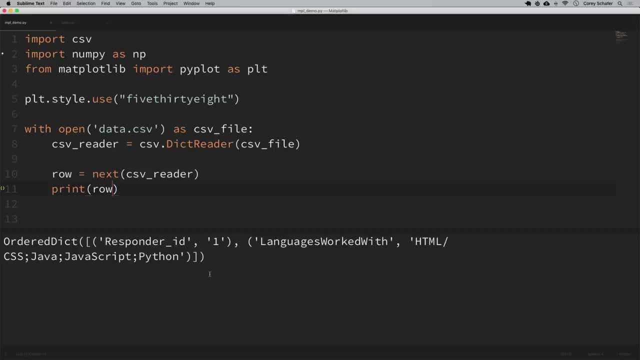 is an order dictionary And the keys are what we saw as the headers and the CSV file And the values are the responses for that particular person. So, like I said, we want to plot the most popular programming languages, So those are within the key languages worked with right here. So 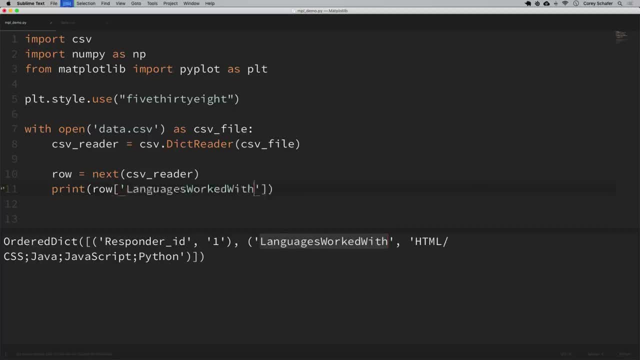 let me just print out that key instead of printing out that entire row. So if I save that and run it, then we can see that now we get those languages And, like I said, these are delimited by semicolons here. So to clean this up a bit and turn this into a list of languages, 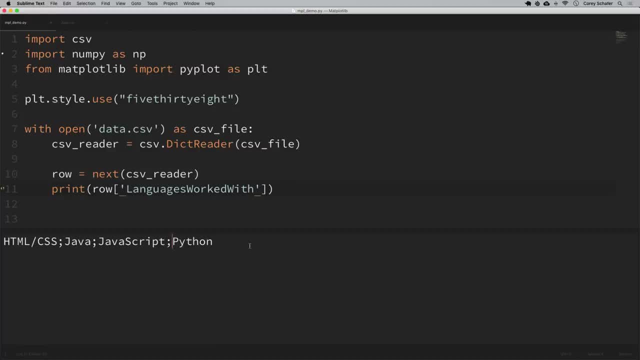 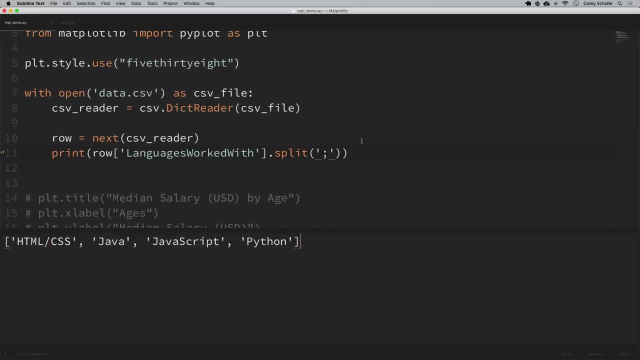 we can actually split the values on that semicolon By saying, after we access that key we can simply say dot split and split on those semicolons. So if I save that and run it, then now we can see that we have a Python list of those languages. So sometimes you're going to run. 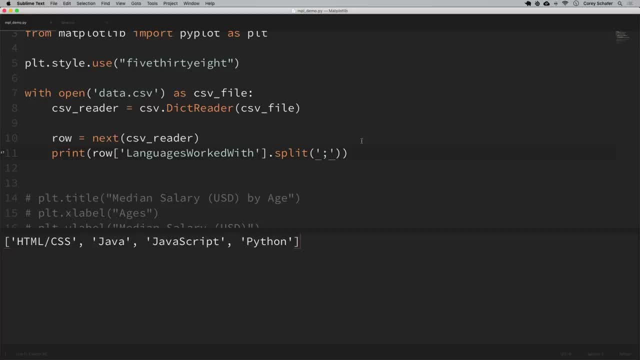 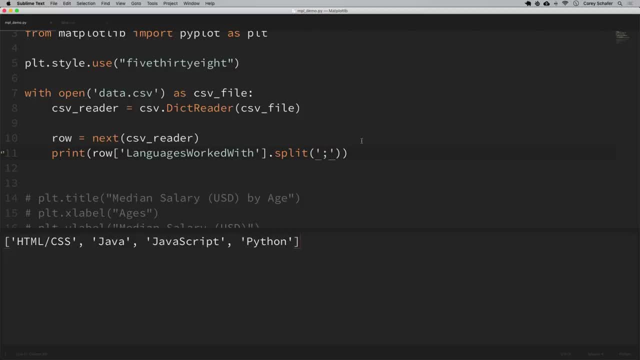 that process here. So in our case we want to plot the most popular programming languages from the results of this survey. So we need to keep a count of each language that each respondent said that they work with. So there are a lot of different ways that we could. 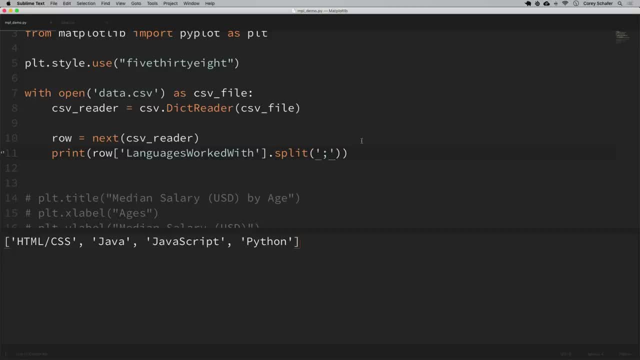 do this as well. We could keep a list and count them at the end. We could keep a dictionary and update the counts of that dictionary each time. But this is actually so common that Python has a built in class for this kind of thing called counter, And it's definitely the best way to do. 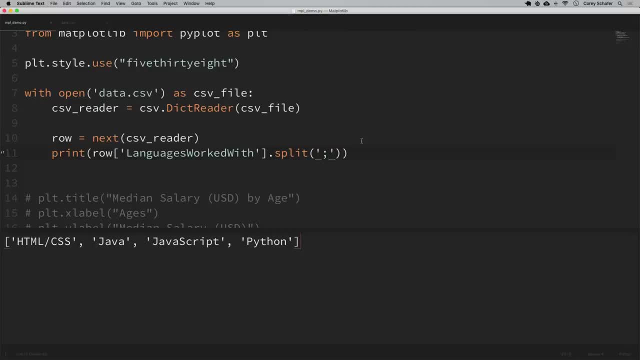 something like this. Now, if you don't know how counters work, they can be extremely helpful, And I plan on making a video specifically about counters in the near future, But I haven't put one together just yet. So first let me show you how a quick example of how counters actually work. So 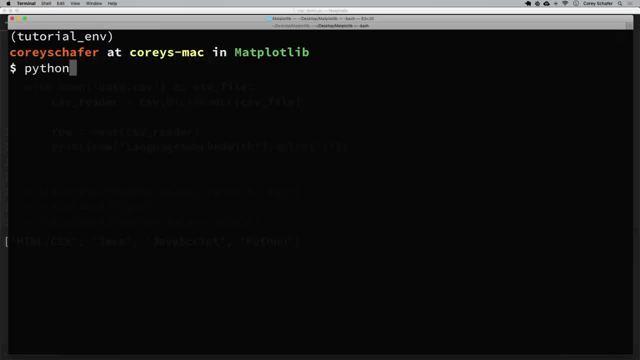 let me open up my terminal here And I'm going to run Python And let me show you how counters work here really quick. So let me open up my terminal here And I'm going to run Python And let me show you how counters work here really quick. So to 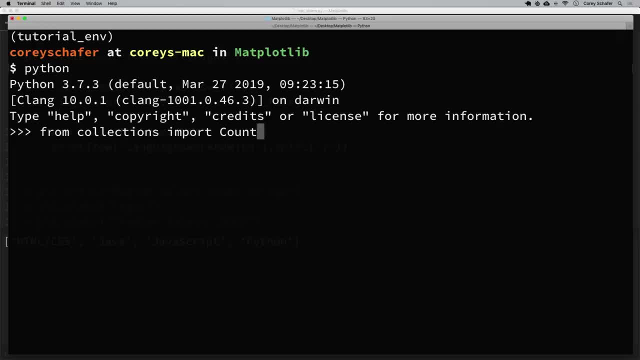 import these, I'm going to say from collections import counter. They are from the collections module And now that we have a counter, I'm going to say C is equal to counter And I'm going to pass in a list here. So I'm going to pass in a list of Python And I'll also pass in a 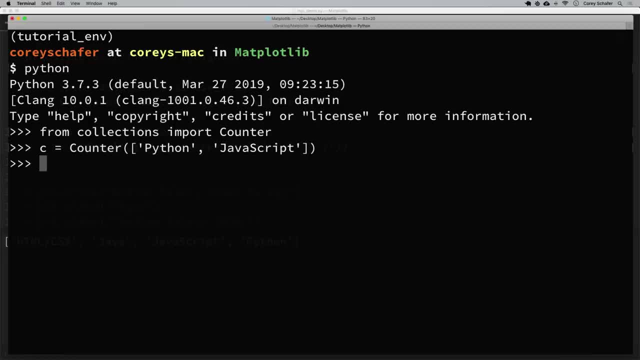 of Python and JavaScript- those two values in my list. So if I look at that counter, we can see that this says: okay, I have a counter here. I have a key of Python And that's currently set to one. I have a key of JavaScript and that's currently set to one. So it's keeping count of how. 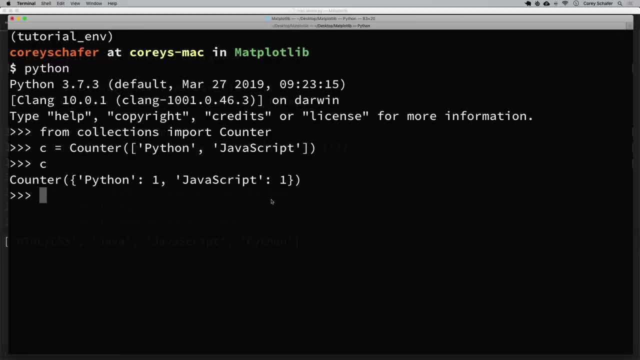 often it sees these values. So to update this counter, I can simply say c dot, update. And now I'm going to pass in a new list. So this new list. let's say this time I say C plus plus, whoops, C plus plus and Python. Okay, so now let me look at this counter. So now, when we look at 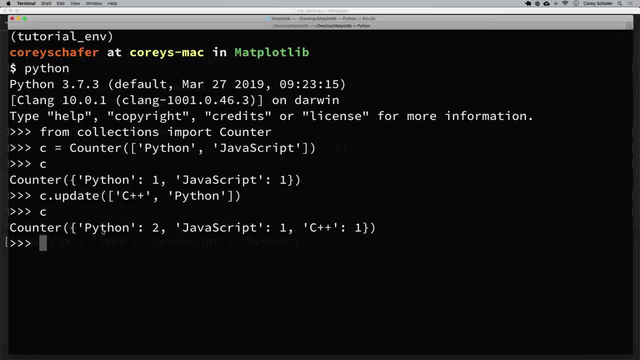 the counter we can see. okay, now Python is two. it's seen Python twice. We saw it up here when we first created the counter and we saw it right here when we updated the counter. It's still only seen JavaScript one time, the first time we 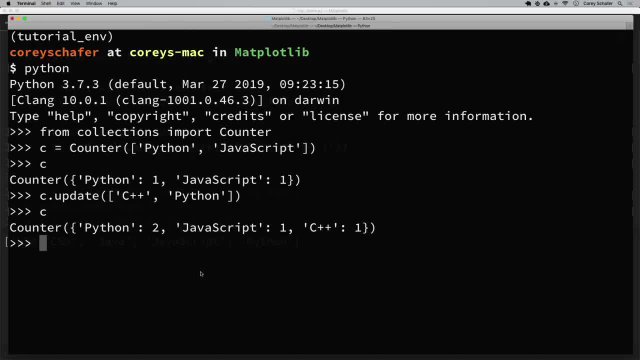 created it and it's only seen C++ one time. So now let's do an update one more time. So if I run that update statement again with C++ and Python and then look at our counter again now it's saying: okay, I've seen Python three times, C++ twice JavaScript once. So this is what we're. 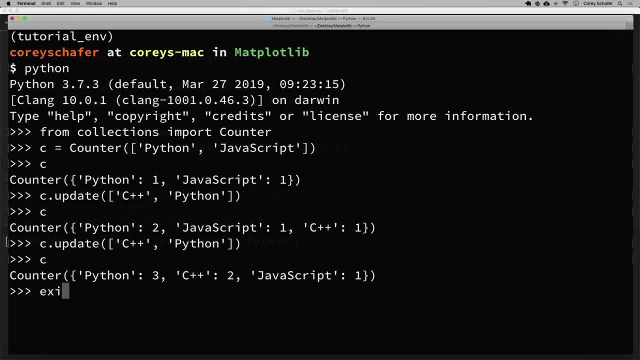 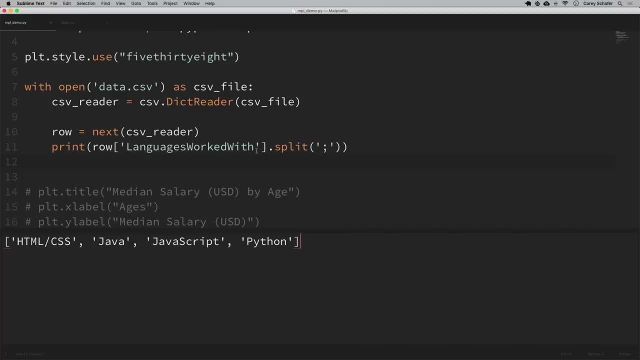 going to use to keep track of these languages. So at the top of my script, let me exit out of Python here. I hope that all made sense to you, because these are the kind of things that you need to do sometimes when you clean up data for plotting. Okay, so I'm going to close down that. 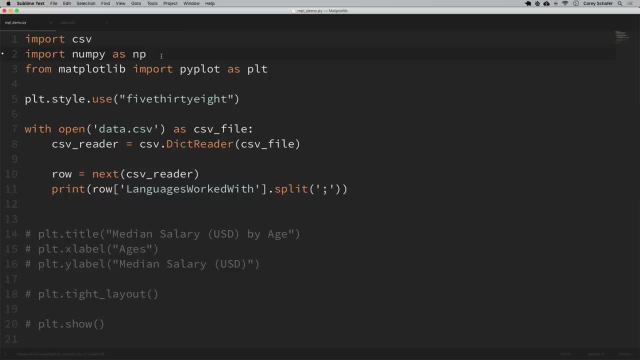 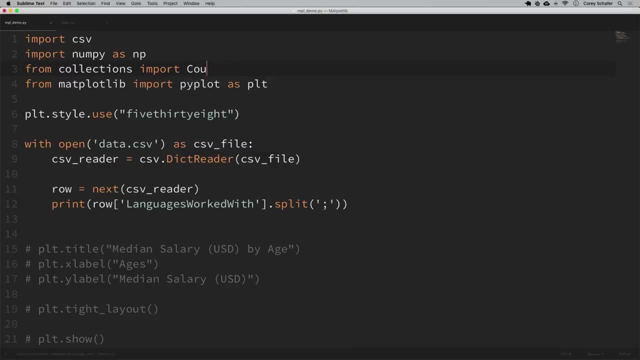 output. Now up here at the top of my script, I'm going to import that counter. So again, that's from collections: import counter. spell that right. Okay, now I'm going to instantiate a new counter. So I'm going to import a new counter. So I'm going to import a new counter. 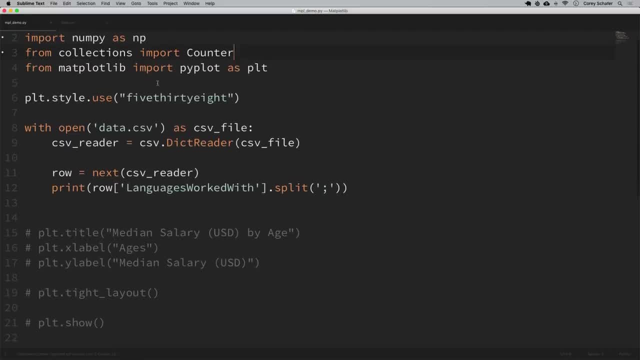 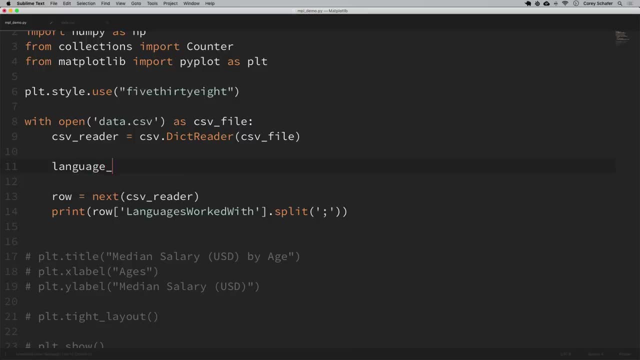 counter right after we read in our CSV data. So right above our row here, I'm going to make a variable and I'm going to call this language underscore counter and set that equal to an empty counter. So right now we only have the data for a single row, but we want to grab the exact same. 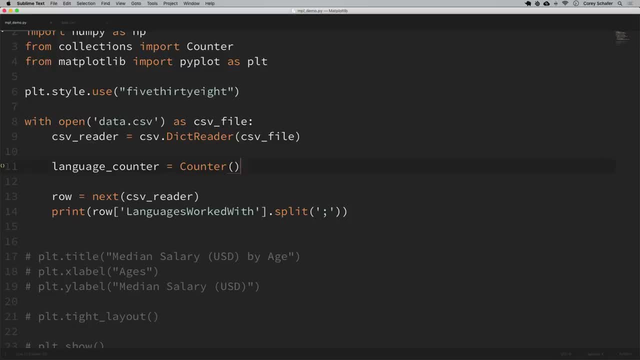 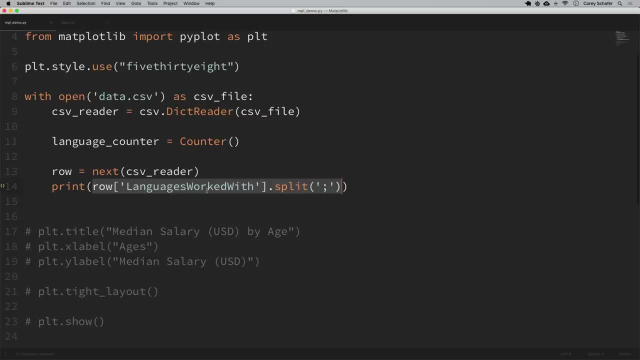 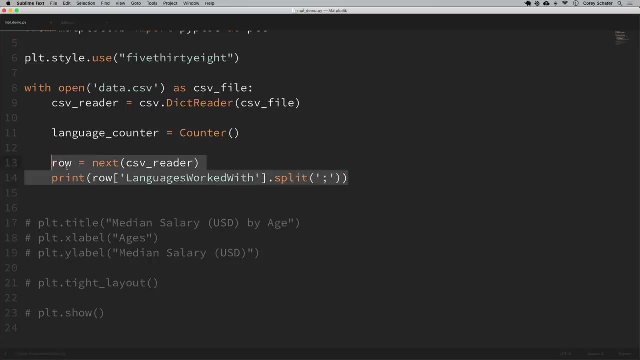 list of languages from every row. So, in order to do this, we can copy what we've already printed out here. This big long thing here is what got us that list of languages from that single row. So let's copy that And now we can loop over all of the rows of our CSV data and update our counter. 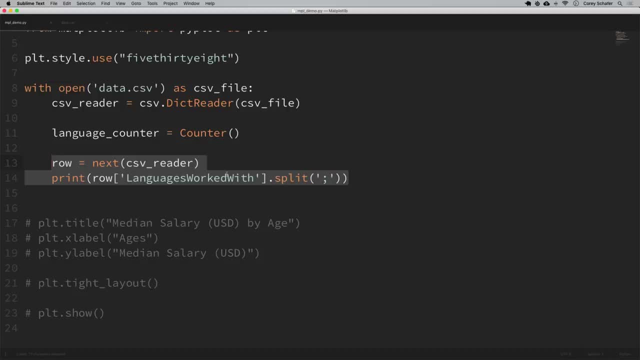 with the data that is within this list here. So I'm going to say for row in CSV reader and this will loop over every row in that CSV file And I'm going to say language counter dot update And we want to update that with the list of languages from every row. So let's copy that. And now we 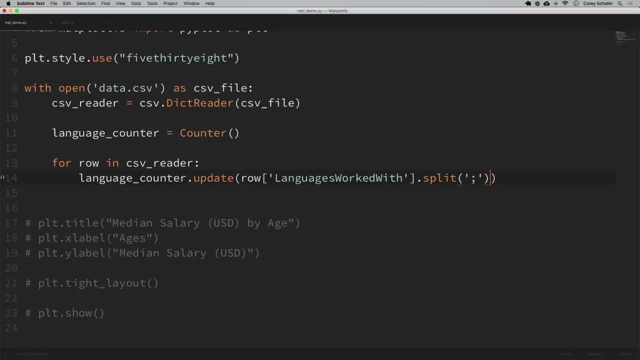 have that list of languages for every single row, So I'm going to paste that in, And this section here is what's going to give us those list of languages. So now our language counter should get updated with all those languages. Okay, so now let's print out our language counter to see if it. 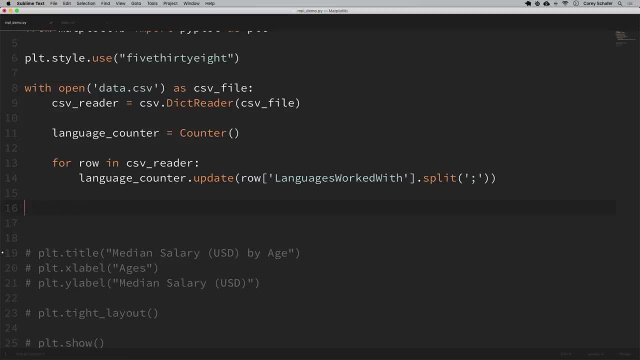 looks like we have some coherent data And I'm going to do this back on the main level of the Python script outside of this with context manager here. So, above our PLT dot title, I'm going to print out language counter dot update And I'm going to print out language counter dot update And. 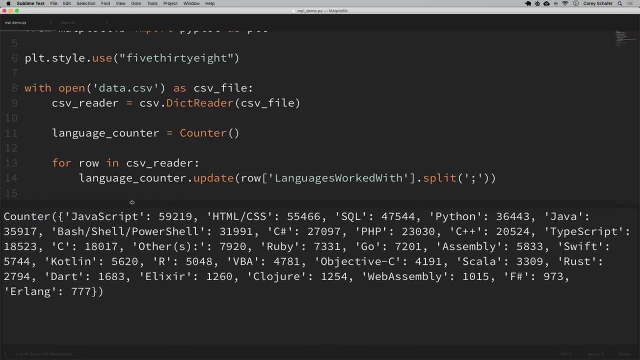 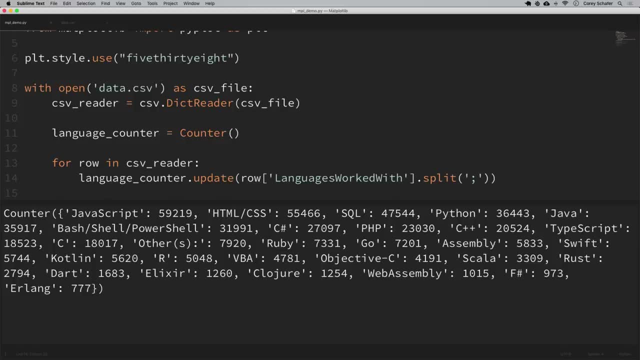 I'm going to print out language counter, So let's run that, And it looks like we've got some good data here, Okay, so, since this is a counter, it should print out sorted with the most responses at the beginning, So we can see here that we have JavaScript with 59,000, HTML CSS 55, SQL 47, Python 36,000,. 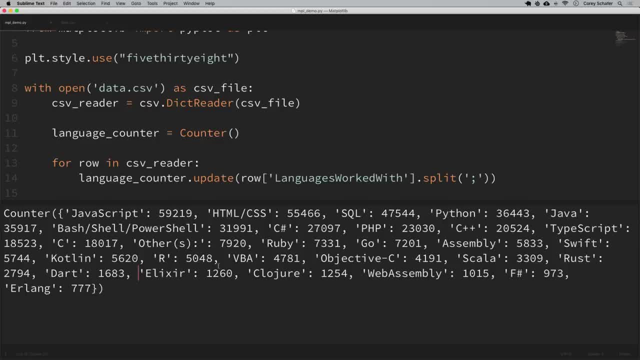 Java 35,000, and so on. Now we can see that there are a lot of programming languages here. If I remember correctly, I think there are 28 total here And I'm going to print out language counter, dot, update And. 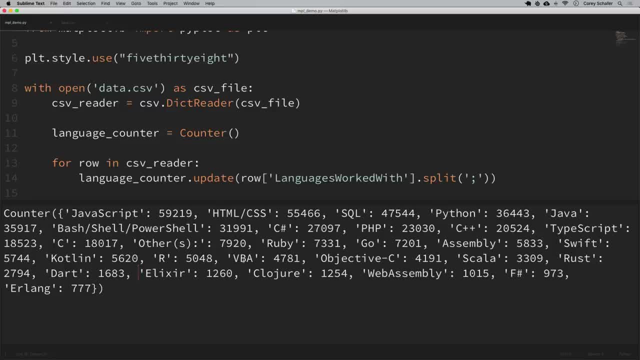 we can see here that we have JavaScript with 59,000, HTML CSS 55, and so on, So we probably don't want to plot all of these. So let's say that we just wanted the 15 most common languages. Well, the 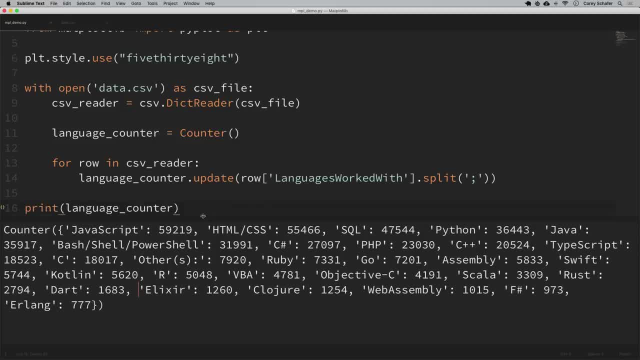 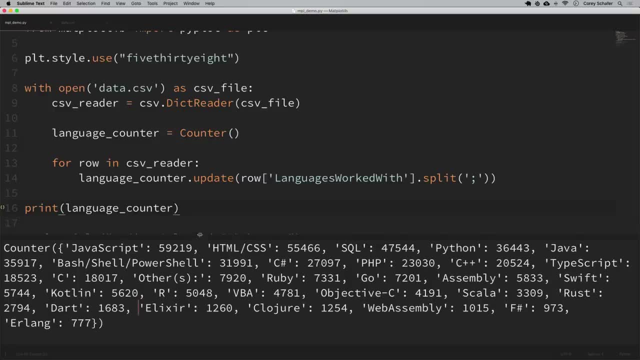 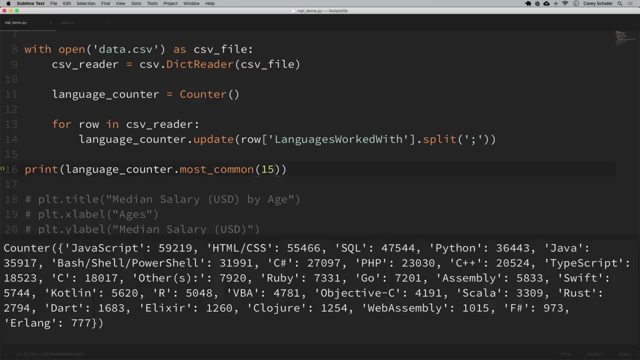 great thing about using a counter like we did here, is that it actually has a most common method built in to do this for us. So whenever I'm printing this out, I could say: print language counter dot most common and just pass in a 15. And if I run that, then that is the 15 most common languages. 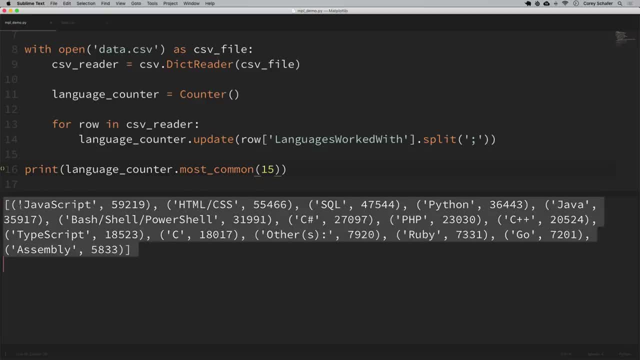 responses, And that most common method actually returned a list here, And each item in this list is a tuple containing. so this is one tuple here. it's containing the language and the count. So now let's try to plot this data. So how would we do this? Well, first we need to split out the 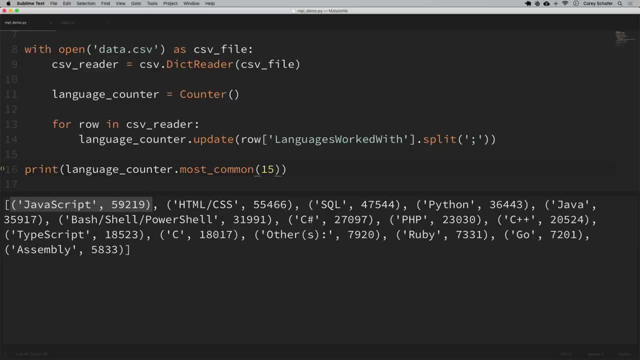 languages into their own list and these corresponding counts into their own list. So when we did our previous bar charts, we had our x and y axis. So we'll want all of our languages on one axis and the counts on another. So that's why we need to split those up. So there are also a couple ways. 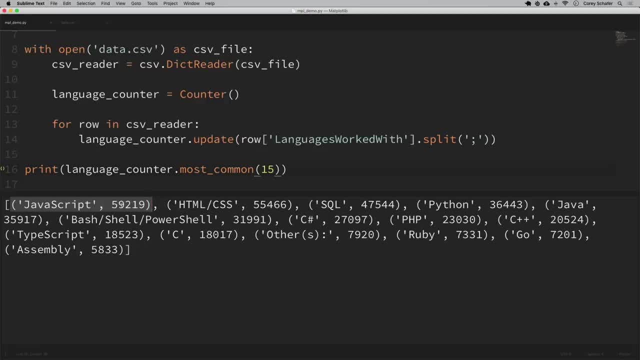 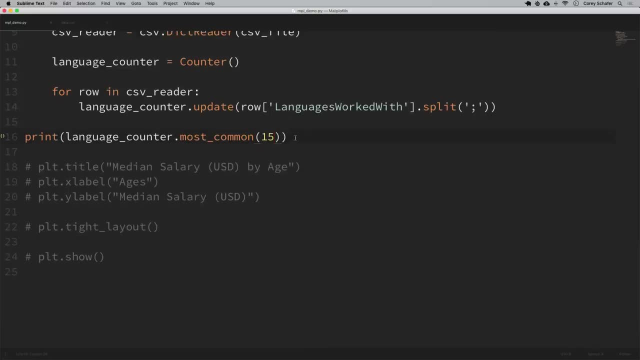 that we can do this. Now let me show you a way that takes a little bit more code but I think is going to be where most everyone will be able to read it. So to do this, I'm just going to overwrite this line here. Actually, I will keep that there for now. But above this line, 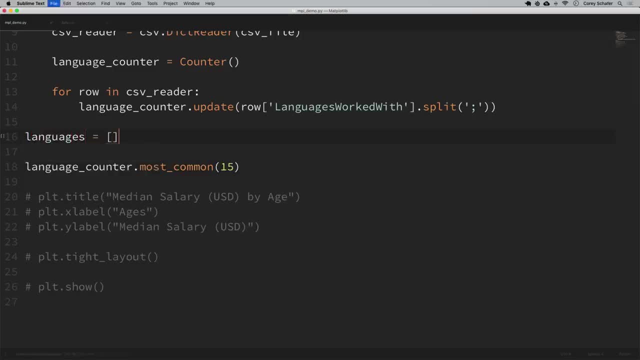 I'm just going to say languages and set this as an empty list, And then I'll say popularity. that's going to be for the numbers. So we want the languages in this list and the corresponding popularity in this list. So now let's loop over all those tuples that we got back from this most. 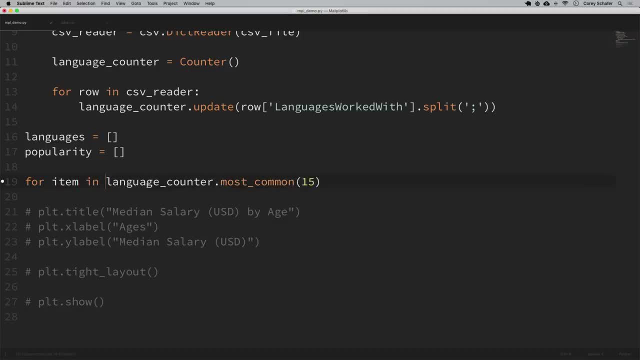 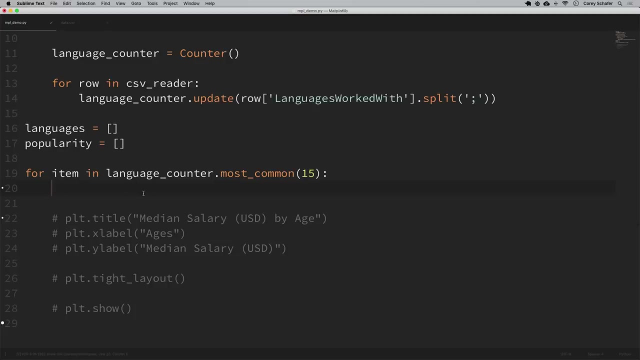 common method. So I'll say for item in language, counter dot most common whoops. and let me sorry, let me go to the next line here And remember this is going to be looping over a list of tuples And the first value of that tuple is going to be the language. 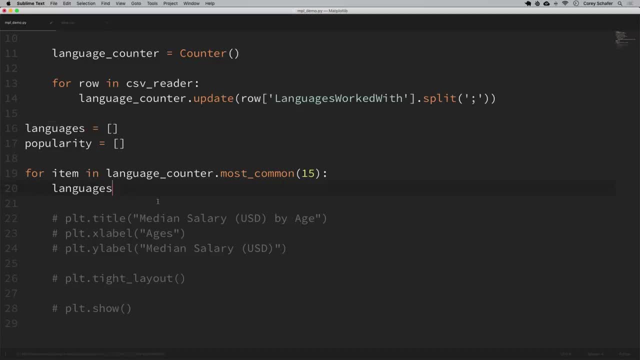 And the second value is going to be the popularity. So I'll just say: languages dot. append item index of zero to grab that first item and append that to our languages, And we want to append the second item to our popularity. So now, if I print out our languages and our popularity, 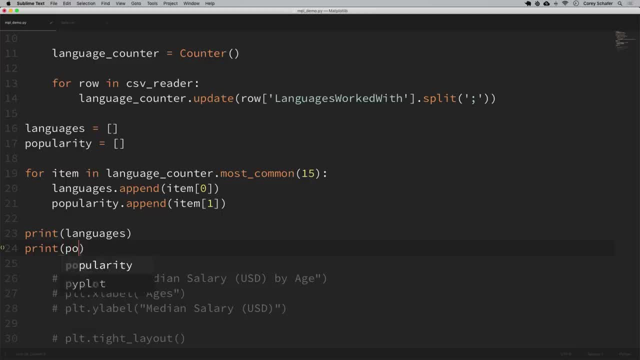 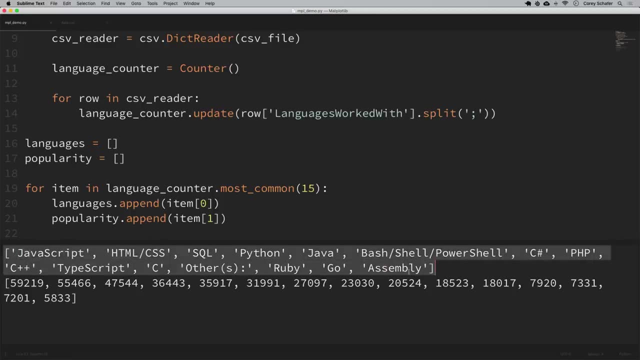 languages, print popularity, save that and run it. then we can see that now we have one list here that is all of our top 15 most common languages, And the second list here is the corresponding popularity of that language according to that survey. So now we can actually use these two. 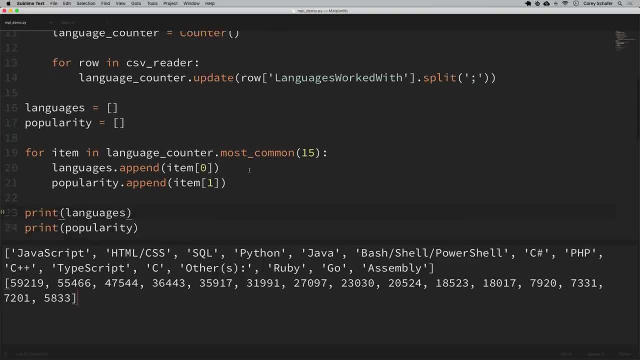 lists for our plot. Now there's actually a way of doing this whole section right here. There's actually a way of doing that with a one-liner, using the zip function and unpacking the list. It's easier to do it in Python that way than through some fundamental accounting. So A 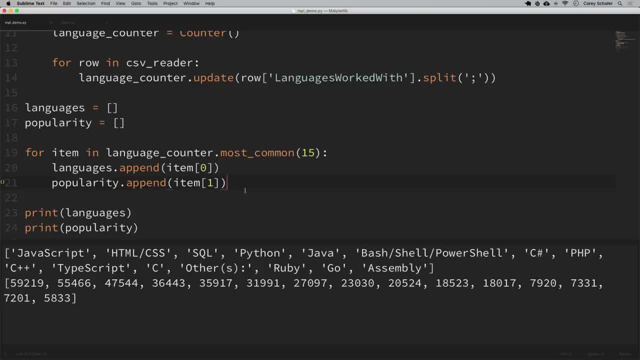 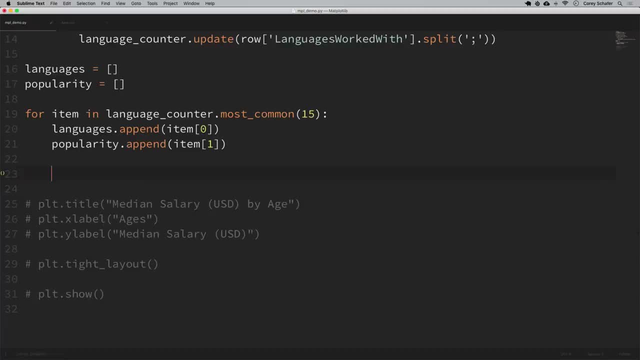 you guys just notice that the list actually has the ainda: any peanut, extra peanuts, some compensate points, some tips, some references and so forth. So there's one browser I only want to use, like the one I've been using, And then I want to create a list And what we'll do is ask for. 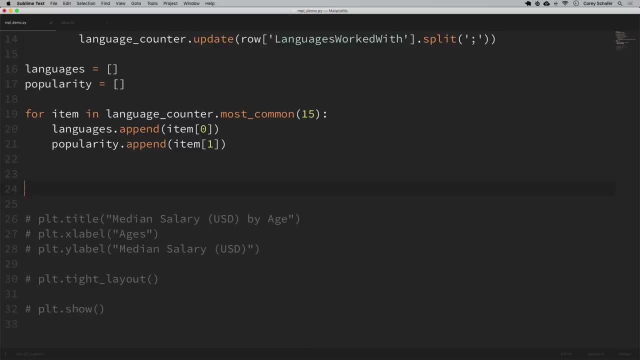 data as well. So we've appeared here in our library And what we do is we get this legal counsel here called pseudo meta, And we've added it And we print that out, And so we see that And we see that x-axis, we're going to plot the languages, And on the y-axis, let's plot the popularity And let's. 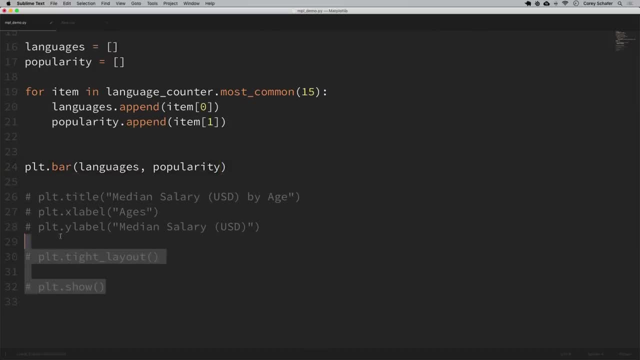 also uncomment out our titles and labels here And let's change those to match what we're actually plotting. So instead of median salary I'm going to type in let's just say: most popular languages Spelled that wrong. That's okay. For the x-label: here I can just say our x-label is the programming. 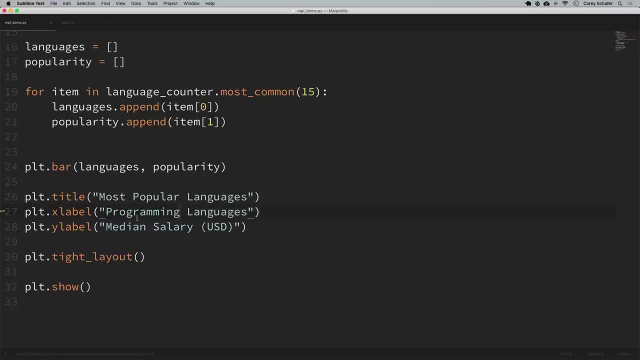 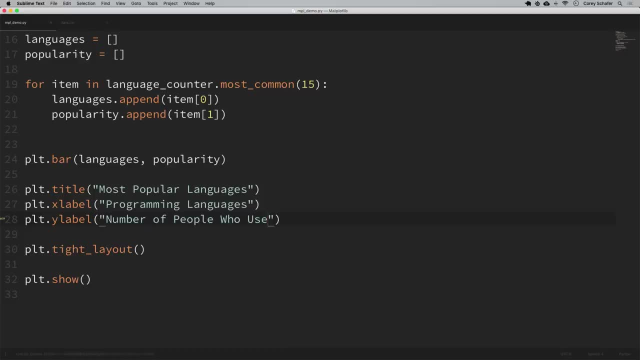 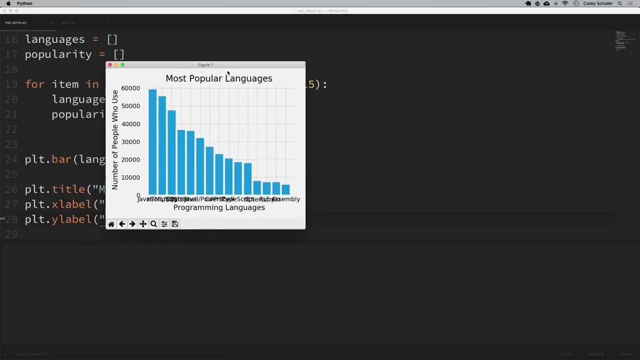 languages. So I'll say programming languages And for the y-label here I'll say number of people who use. Okay, so now, with that in place, let me save that and run this. And let's take a look at our chart. Now we can see right off the bat: when we have this many items, it's hard to 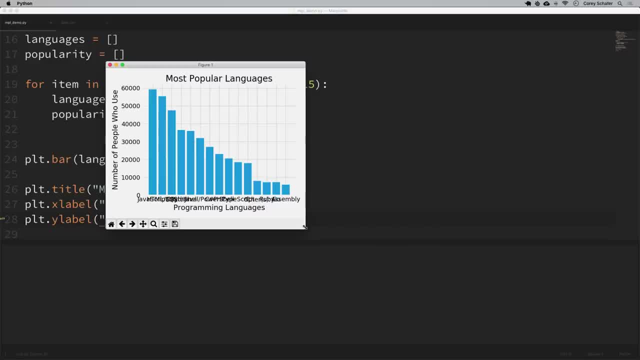 see all of these using a vertical bar chart, like we did here. When you have a lot of items, then it might be more readable to use a horizontal bar chart. So let's take a look at our chart Instead, and we can do that easily just by changing our bar method to a bar H method. So 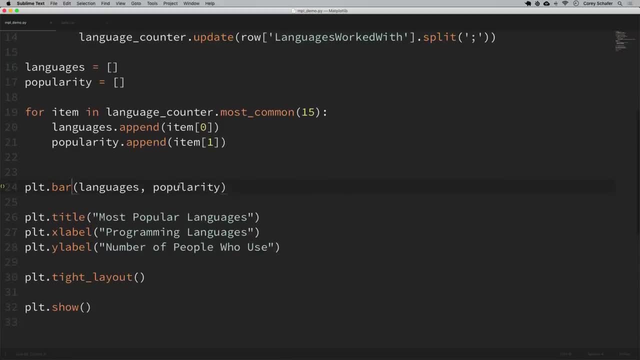 right here where we're saying dot bar. I'm going to change that and say dot bar H. So now we can leave our arguments exactly as they are, because the horizontal chart expects the y-axis values first, So we'll just keep our languages there. Now we will have to change our axis labels here. 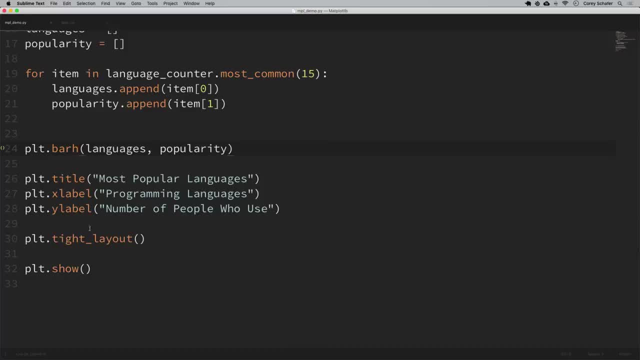 because those are going to be different now. So I'm just going to switch The x and y labels here real quick. So I'm just going to have programming languages as our y label, number of people who use as our x label. Okay, And now I think that's about it, And 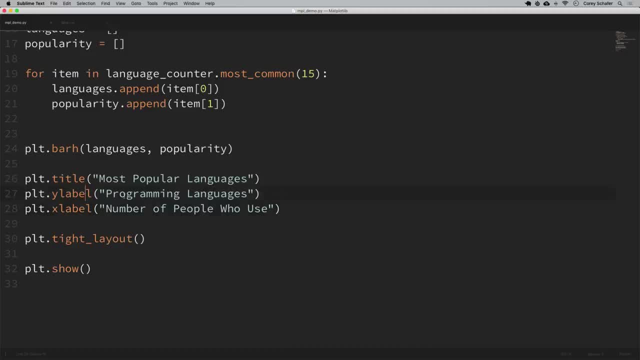 actually, now that I think about it, I don't even think that we need this y label telling us that these are programming languages. That's pretty self-evident, since the names of the programming languages are actually the labels themselves. So I'm just going to get rid of that. That's one. 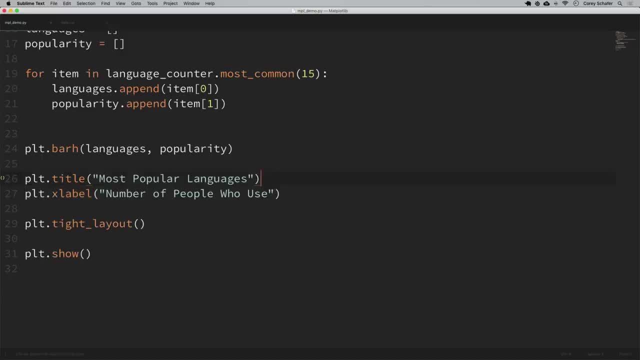 thing with plots is, it's nice to be descriptive, but you can also be overly descriptive, So I'm going to get rid of that. Actually, just let me comment it out instead. Okay, So now let me run this. and now we can see that we have, oops, a vertical bar chart here. Let me open this back. 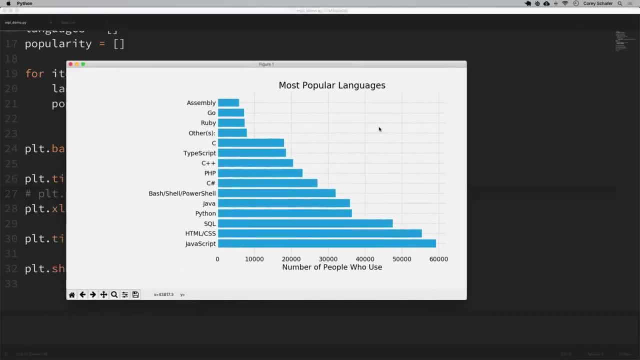 up, make this a little larger, Okay. So what I meant to say is we have a horizontal bar chart here, So we can see that this is much easier to read with a lot of values and that those aren't scrunched together like they were in that vertical bar chart. So whenever you're plotting things out, 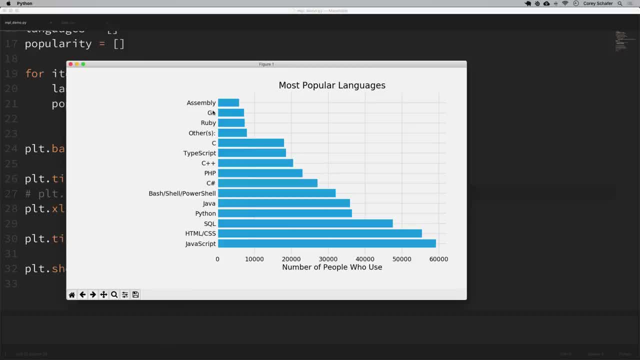 if you've got a lot of values to plot- you can see that you've got a lot of values to plot With a bar- then it might be a good idea to use a horizontal for this type of thing. Now, one thing here is that with a horizontal bar chart, maybe you want the most popular language. 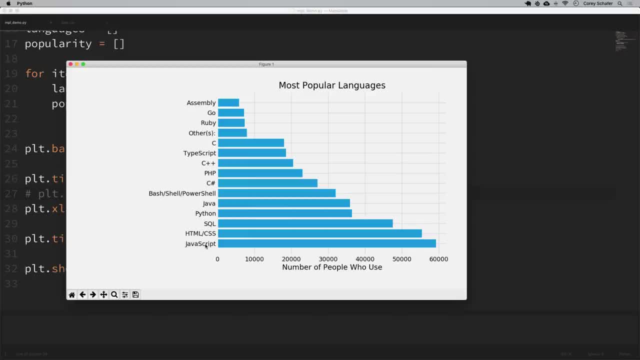 right now it's down here at the bottom. Maybe we want that at the top, since we read from the top down. So to do this, we could simply just reverse the list that we're passing into the bar H method before we actually plot it. So I'm going to close that down And now up here before that bar H. 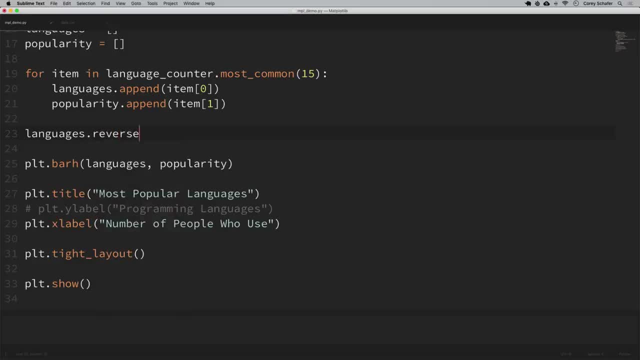 method. I'm simply going to say languages dot Reverse and popularity dot reverse, And the reverse method on a list actually reverses those in place, So we don't need to set languages equal to this or anything like that. It's actually going. 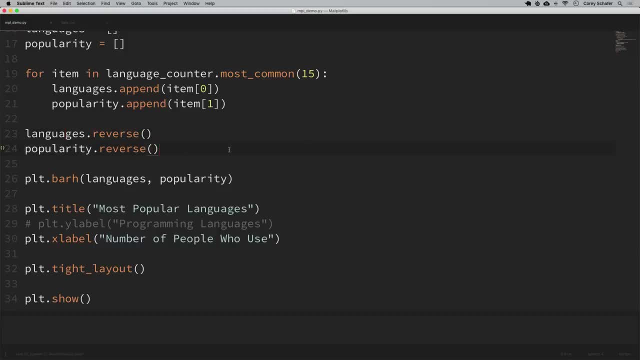 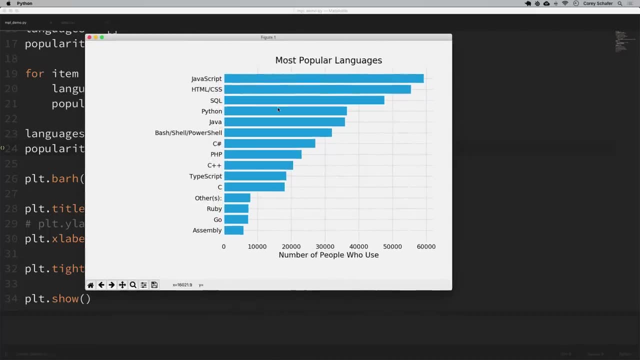 to modify that list in place. So now, if I save that and run it, then now we can see that we have the most popular languages up top And I think that that looks a lot better Now. I did say that I was going to show you a faster way to load in that data from the CSV. 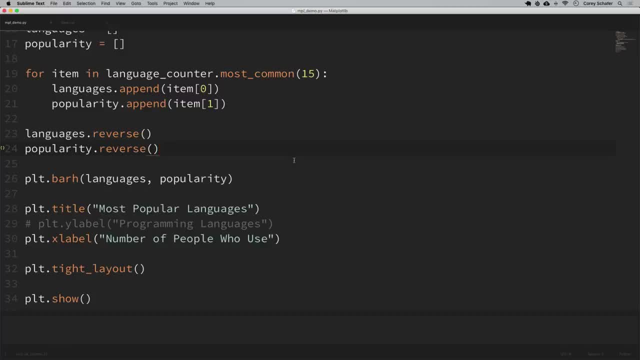 So let me show you how to do that, because for the rest of the series I'm probably going to use pandas to load in data, since it's a bit faster and it's also a bit cleaner. So, first of all, if we don't have pandas installed, then we'll need to do that, And it's really easy to install. So first, 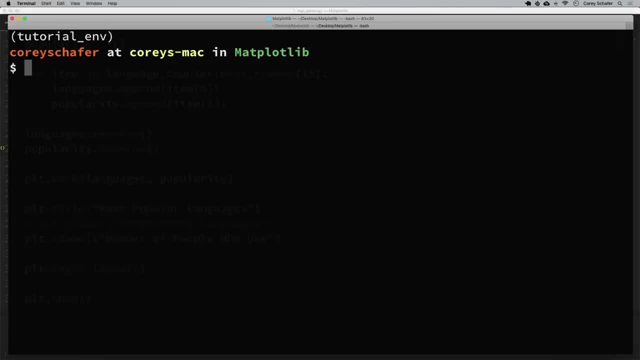 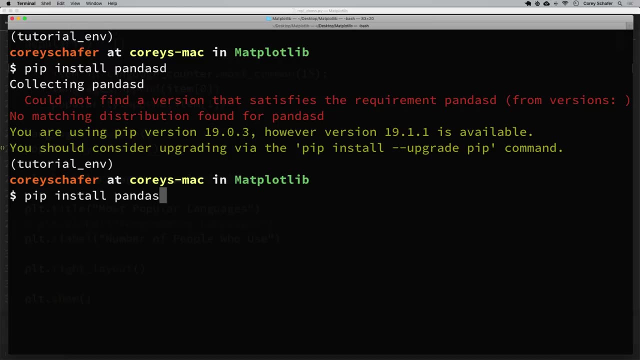 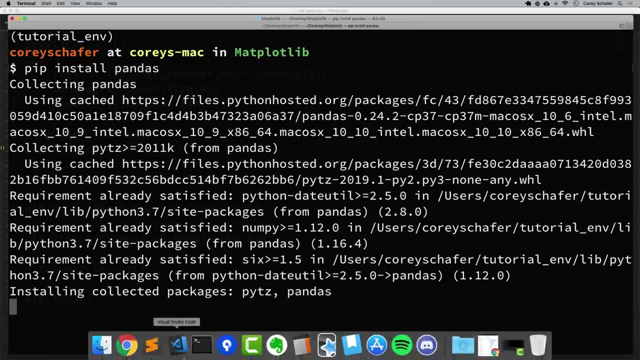 let me install that. I'll just open up my terminal here and clear this out. And we can just install that using pip by saying: pip install pandas. Whoops, got the wrong spelling there: Pip install pandas. And now, once that's installed, we will need to. I'm just going to assume that that. 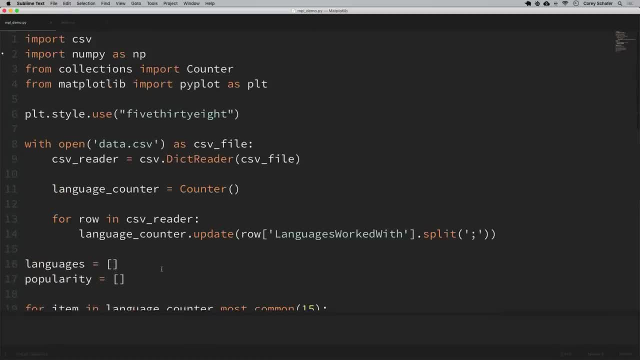 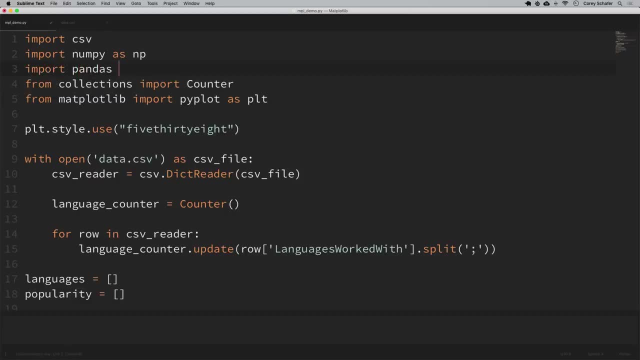 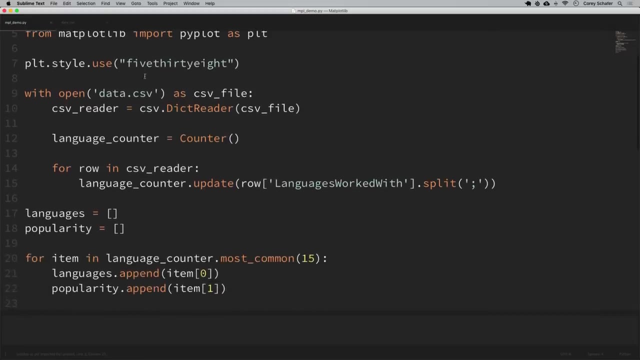 installs correctly and it did. Okay. So back here in our script, up here at the top, we need to import this. So I'm just going to say: import pandas as PD. That's another convention when you're using pandas is to import it as PD. Okay, So up here at the top of our file, instead of opening our file. 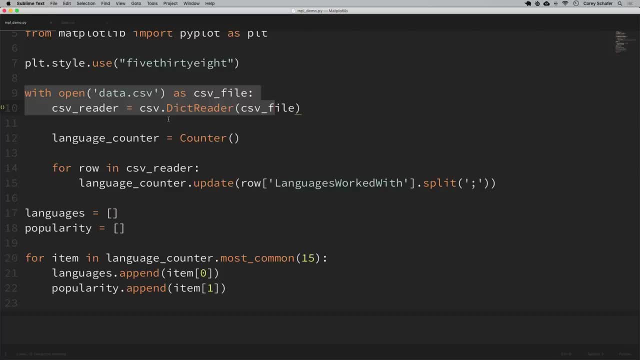 and using the dict reader method to read in the data. we can instead replace that with a pandas method. So now, instead of doing it like this, we can simply say: so, I'm going to get rid of this with context manager here. And since we 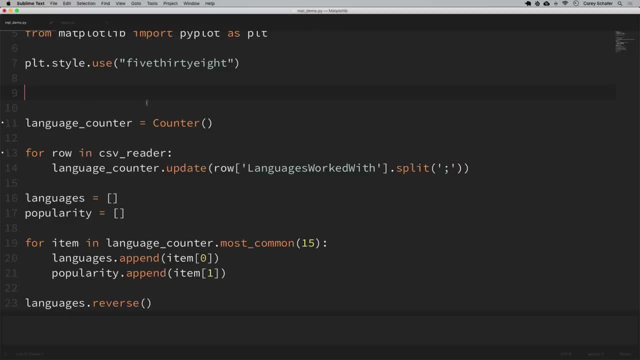 got rid of that context manager. I'll unindent these other lines here, But now where we were opening that file, instead I can simply say: data is equal to PD dot. read underscore CSV and pass in the name of that CSV file. And it was data dot CSV. 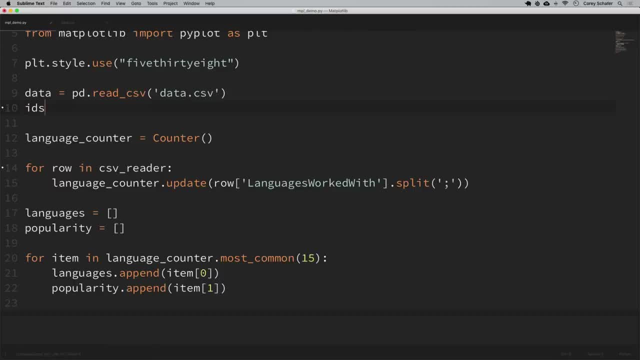 And now I can specify some columns. So I'm going to say that the ID I'm going to create this ID's variable and I'm going to see ID is the- let me see exactly what that column name was- responder ID. So I'll pass in responder ID there. So that's going to set this ID's variable equal to all of. 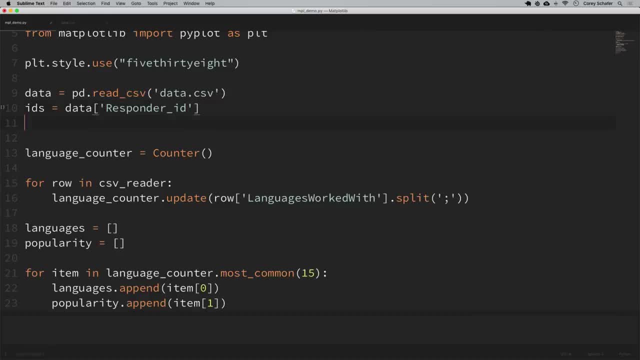 the IDs in that responder ID column And we can do the same thing with the languages. So I'll call this variable Lang underscore CSV, So I'm going to pass in responder ID there. So that's going to set this variable Lang underscore. responses is equal to data And we want the key to be languages. 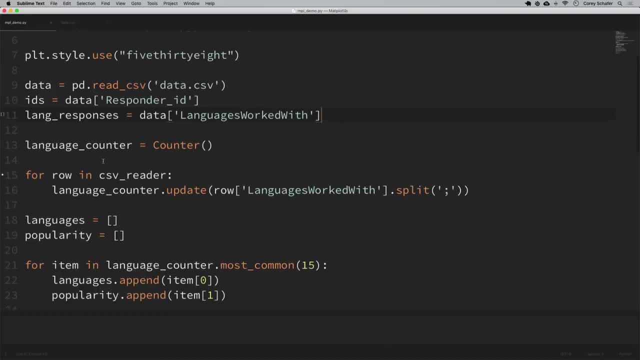 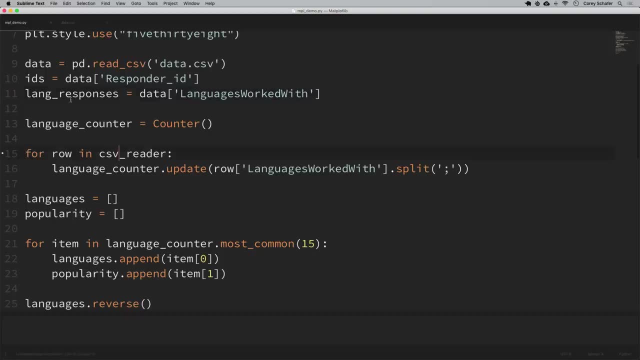 worked with, So I'll grab that. So we still want our language counter, but now here for our loop, instead of saying for row and CSV reader, this doesn't exist anymore. Now we have this list of languages here, So I can just say for response in Lang: responses: update that counter. So the 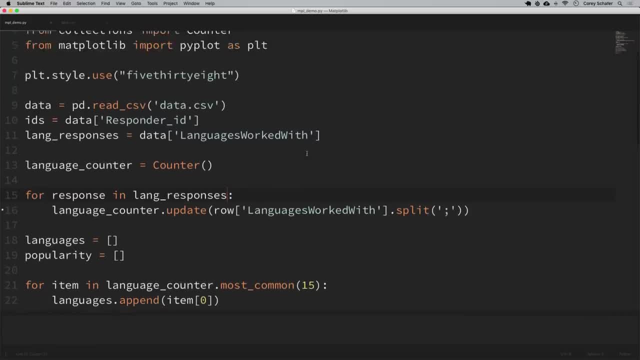 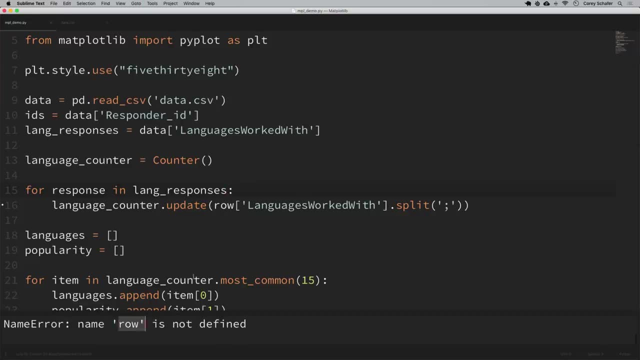 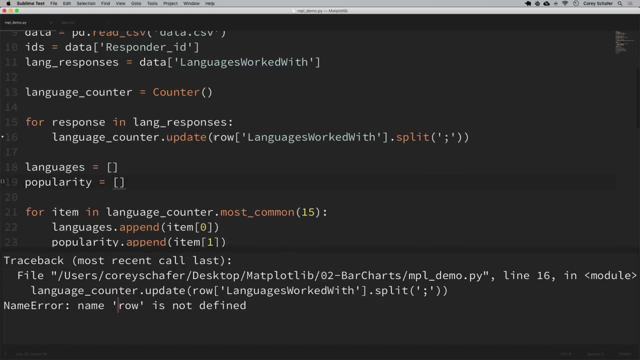 simple update to our code. there should work exactly the way that we that it worked before. So if I save this and I run it, then, whoops, name row is not defined, Okay. So yeah, I got an error here that says name row is not defined. I also meant to update this section here because there's 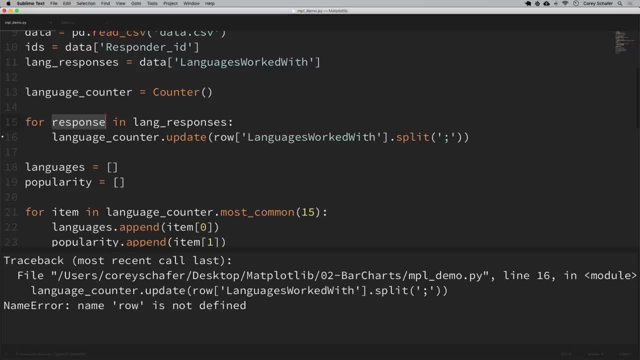 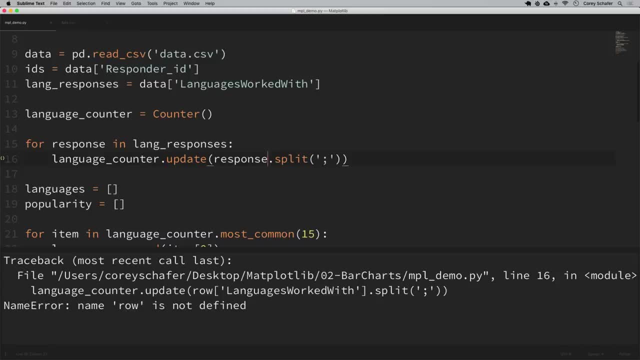 no row anymore, So we just want to split the response instead. So response dot split, because remember these Lang responses here when we're looping through these, each response is going to be this entire section here of all of the languages, So we can simply. 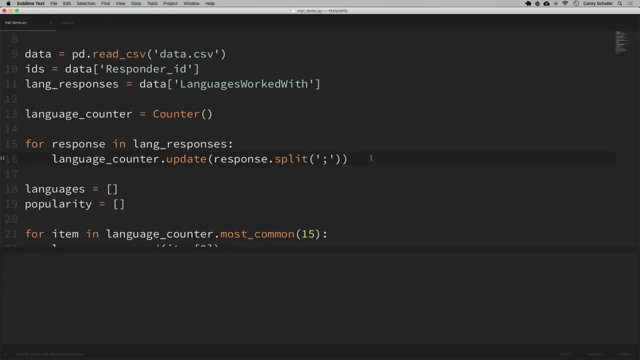 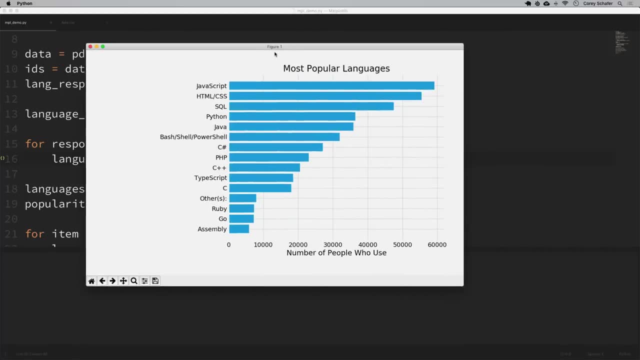 just split that response. Okay, So I'll save that and run it And this should work exactly like it worked before And we can see that it does. That looks pretty good. Now, like I was saying before, this is actually real world data that I grabbed from their actual survey And I 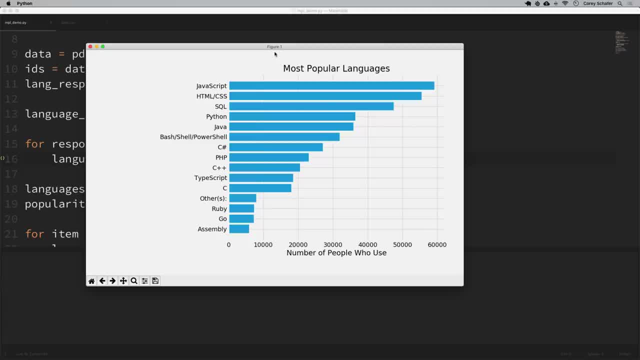 actually have those charts that Stack Overflow put together when they analyze their survey data. So let me open those up and see if we got similar results. So I'm going to put in here. I'm going to put in here. I'm going to put in here. 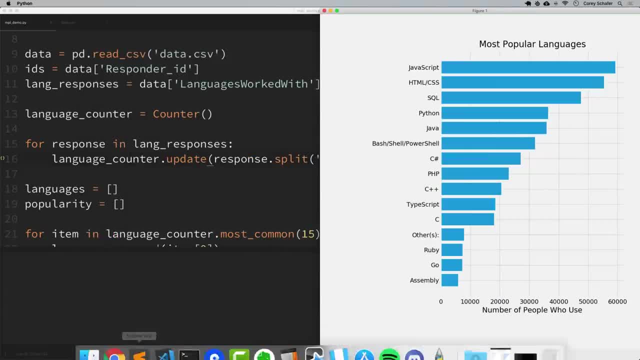 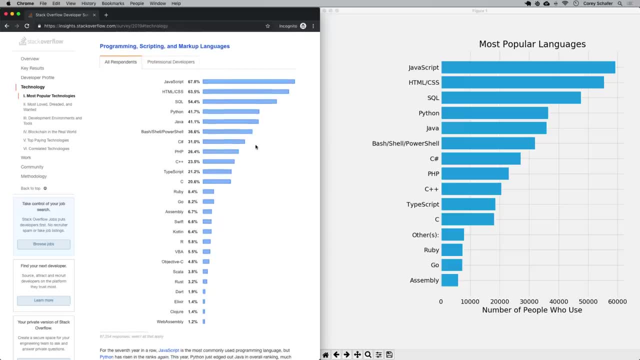 I'm going to put my chart here on the right and their chart I have open here in the browser, So let me open that up. Okay, So here is their chart plotting out the exact same thing that we just plotted. Now there could be some small differences here based on how I sanitized the data compared to 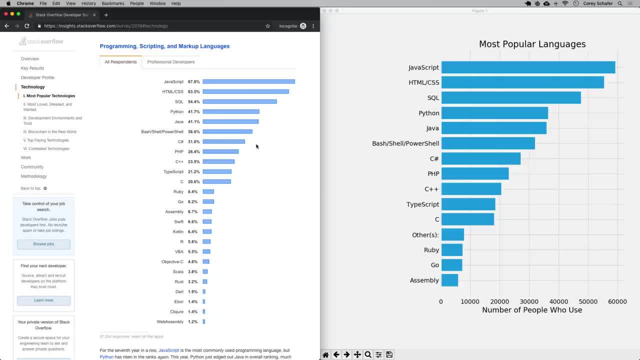 how they sanitized it, But you can see that, as far as the order goes, we got the same results. They've also styled their plot a bit further, but with a little customization we could probably get something very similar. So it looks like we're going to be able to get a little bit more. 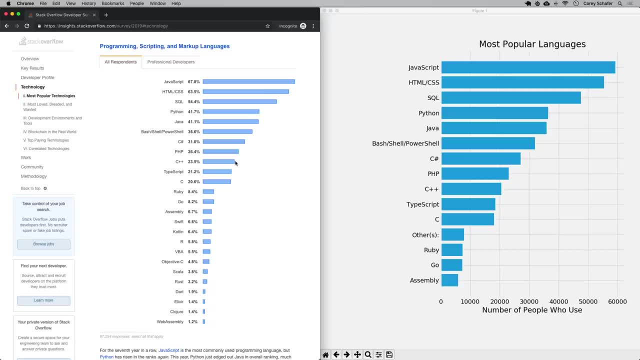 different, with just a couple more different colors. So let's just add in a little bit of spacing and also make these lines a little thinner, and it would almost be identical. So that's why learning things like this can be extremely useful, because these companies are 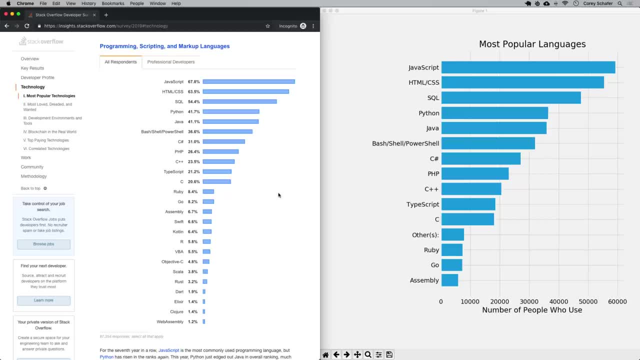 constantly looking for people who can analyze their data and present it in ways that can give insights like this. So this is definitely a skill that you're going to be able to apply to a lot of different situations, just like we did here. Okay, So before we end, I'd like to 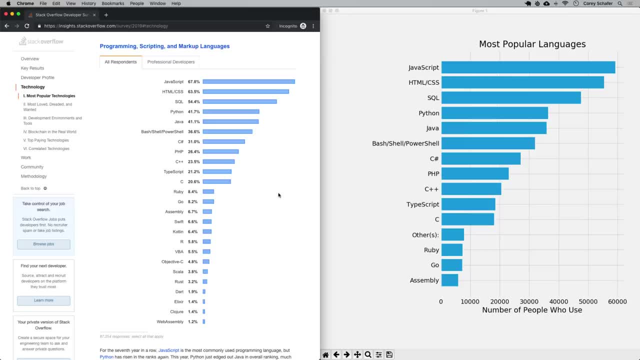 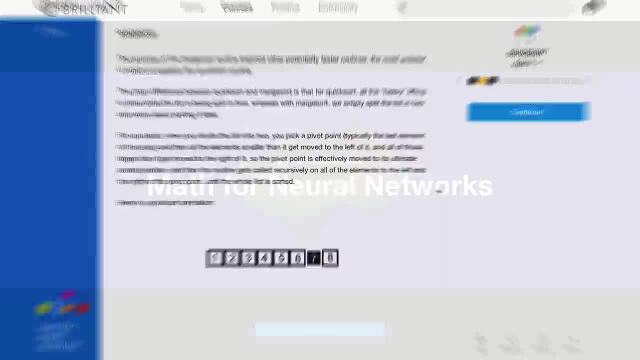 mention the sponsor of this video, and that is Brilliantorg. So if you're interested in this, Brilliant is a problem-solving website that helps you understand underlying concepts by actively working through guided lessons. They have computer science courses ranging from algorithms and data structures to machine learning and neural networks. 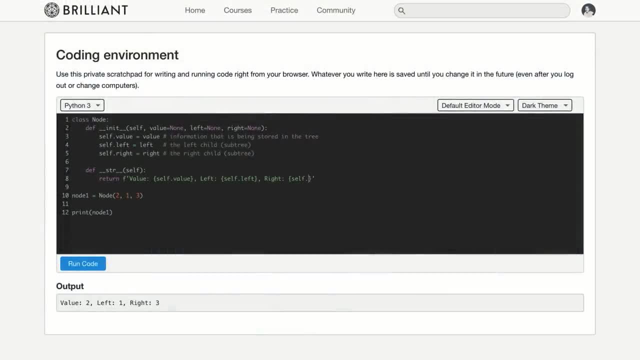 They even have a coding environment built into their website so that you can run code directly in the browser, And that's a great way to compliment watching my tutorials, because you can apply what you've learned in their active problem-solving environment and that helps to solidify that knowledge.